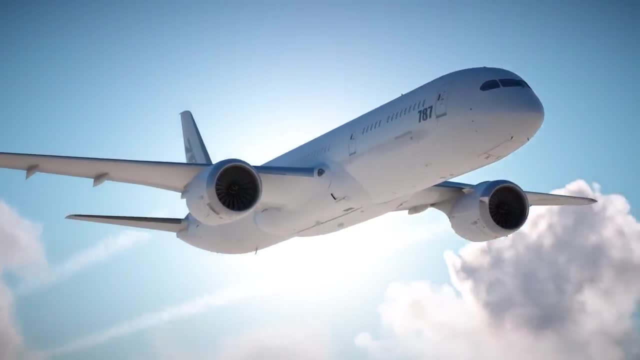 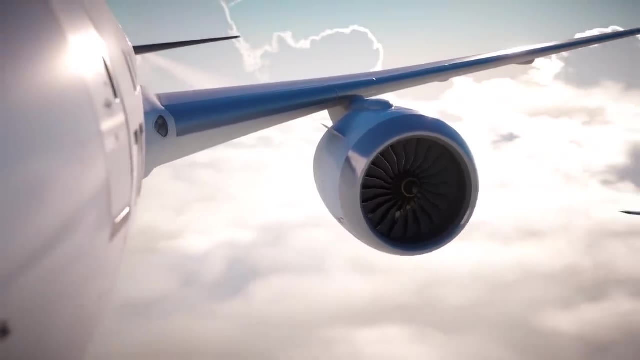 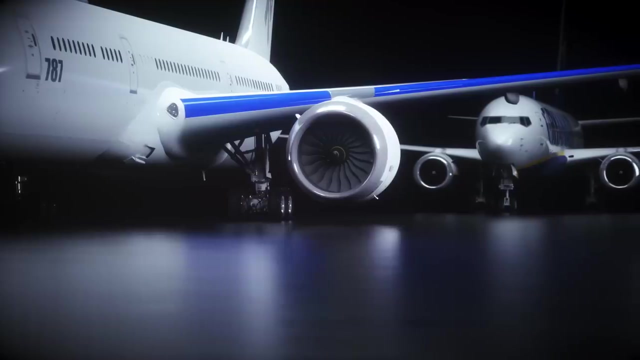 atomic structure of metals to create turbine blades that are actually one single crystal, to delicate robotic machining that humans could only have dreamed of a decade ago. The jet engines of today are barely recognizable to those of the 1940s. They're bigger, they're more powerful and they're more efficient. 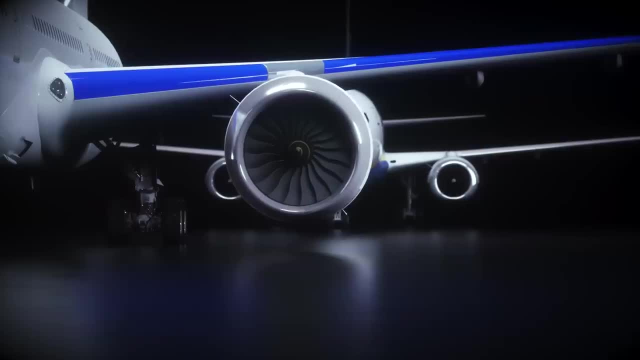 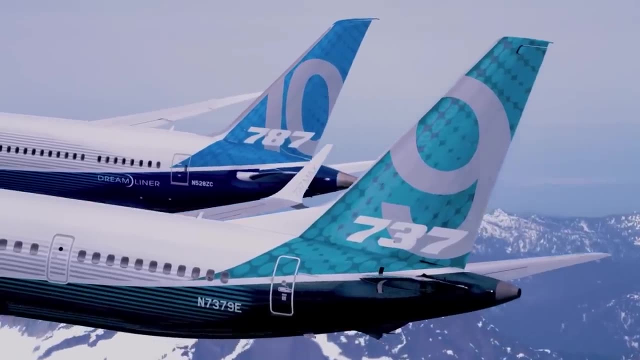 The Dreamliner's engines are so big that they are the same diameter as the 737 fuselage, And this is just part of the puzzle that has allowed the 787 Dreamliner to break world records In March 2020, in the midst of a global pandemic. 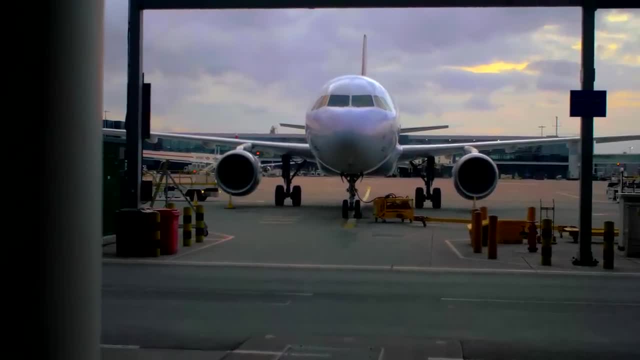 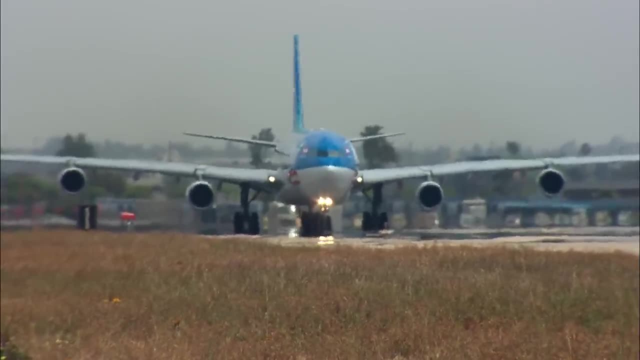 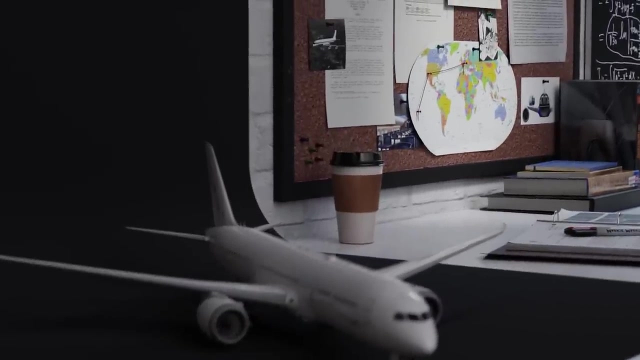 the US government imposed travel restrictions on all of the jet engines of today, All European travellers, A move that cut off France from one of its far flung territories in French Polynesia. Business as usual for Air Tahiti was no more. A creative solution had to be found to replace their regular flights between: 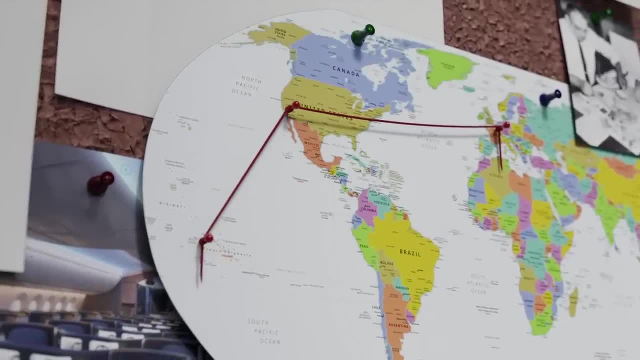 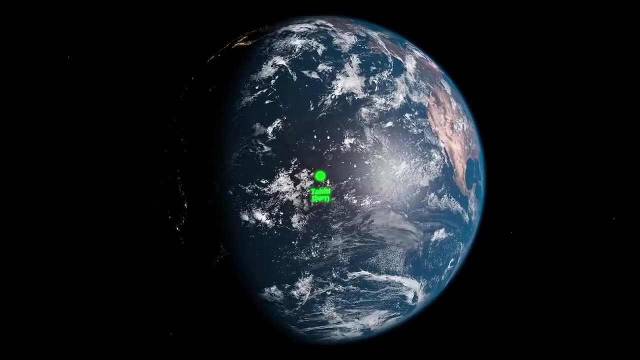 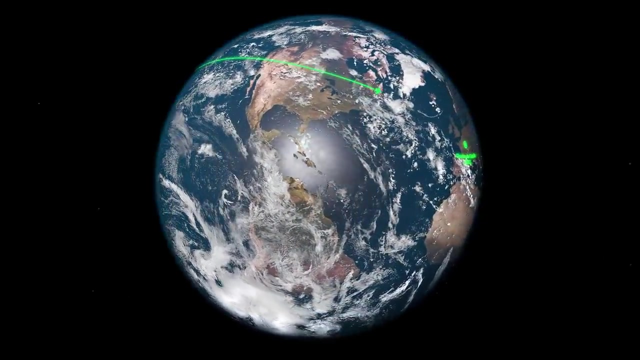 Tahiti International Airport and Charles de Gaulle Airport, which, under normal circumstances, stopped over in LAX Faced with disruption, Air Tahiti began operating the world's longest flight: A 16 and a half hour, 15,700 kilometre, non-stop flight between Tahiti and Paris. 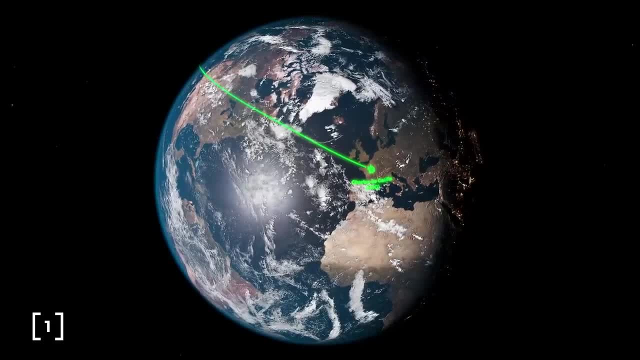 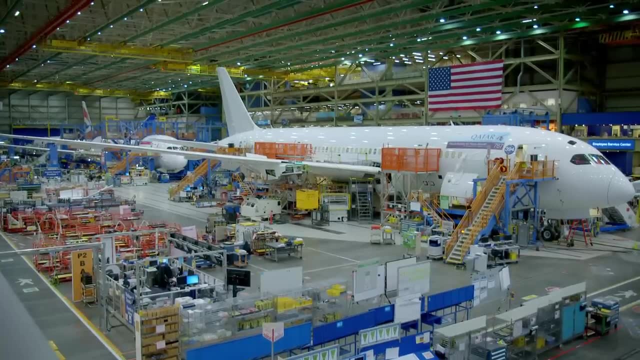 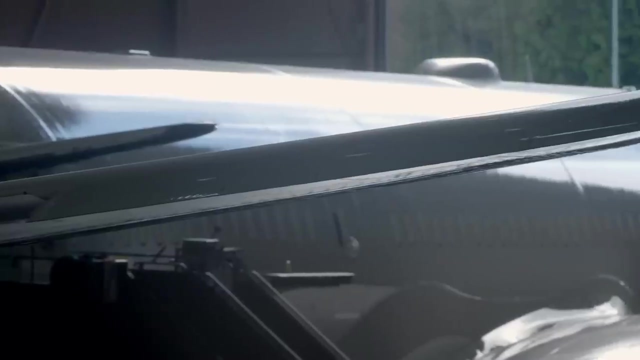 The world's longest distance scheduled flight And it was technically a domestic flight. The 787 made that possible and today we are going to learn how. In our last video, we explored the incredible engineering that has gone into sculpting the airframe of the 787. But all of that work is useless without a power system to operate. 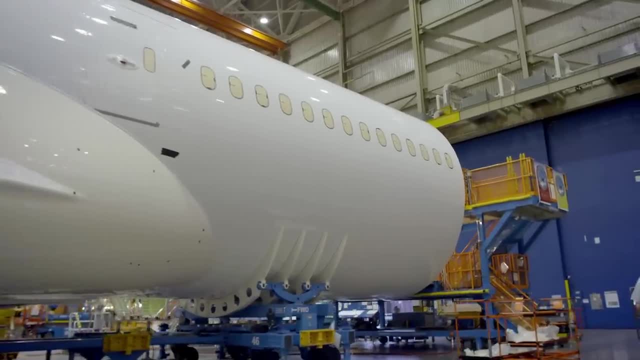 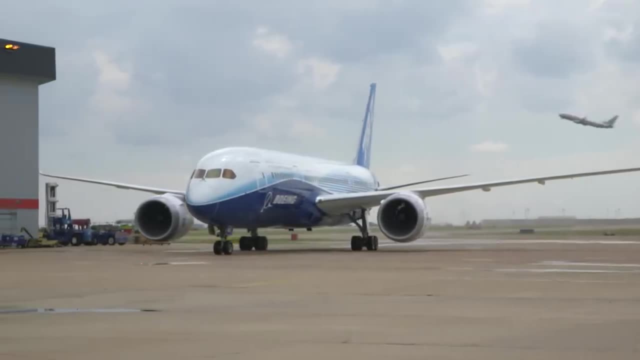 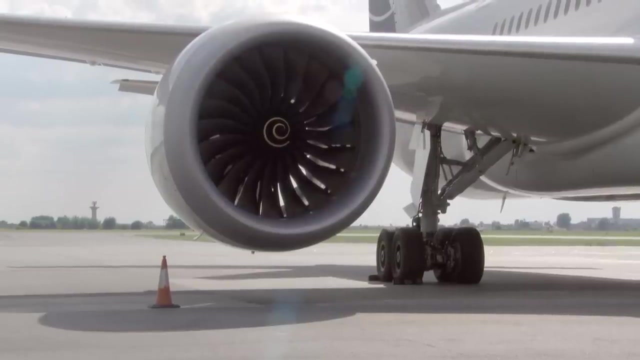 The simple thing we are going to learn isn't to have the永list system with Air Tahiti. that is the only home fighter for the AI approach. We need to get the compressor section turning in order to achieve adequate compression for engine ignition. So if you were to want to know how theflight has been suitable, 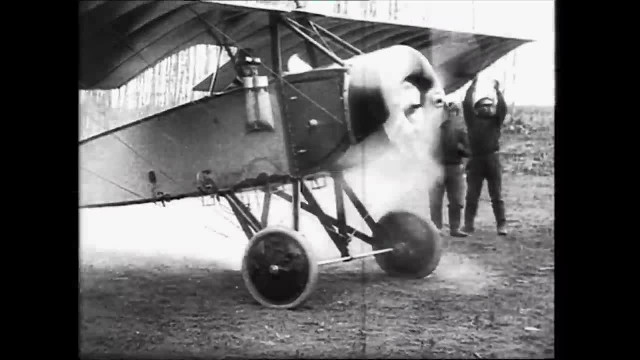 you should check out SOTIE at the current episode of SOTIE, where you can learn exactly what happened. Finally, frankly, what has we during the 7.5 multiply alone flight is them, but we will cover it later. This obviously isn't feasible for jet engines. 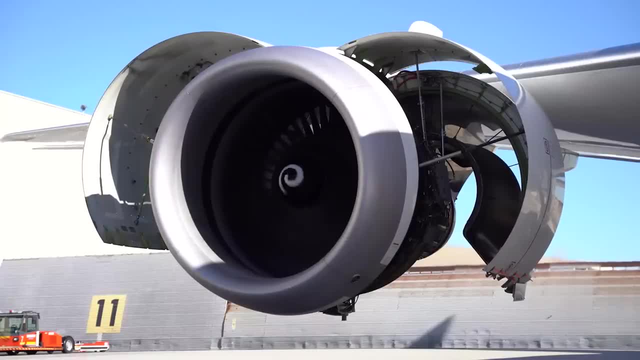 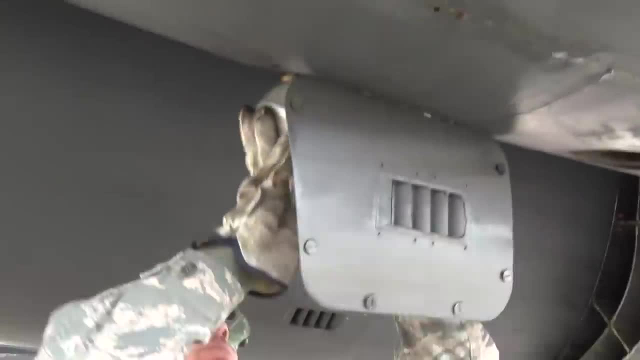 Meaning air 파 outta class is now full, Not fresh Guinness- Do we know what's happening? which need to rotate at very high speeds to start? Engineers have dreamed up many ways to complete this job. Some engines use explosive cartridges that look like shotgun shells that will be fired. 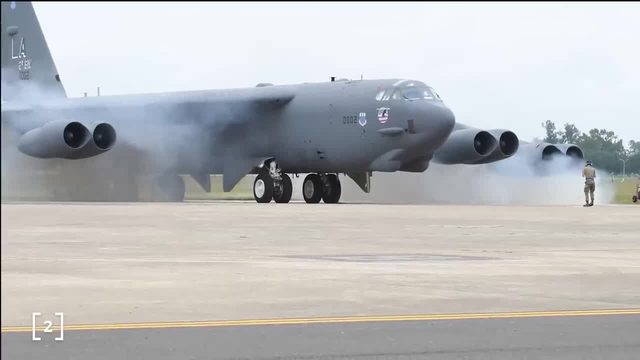 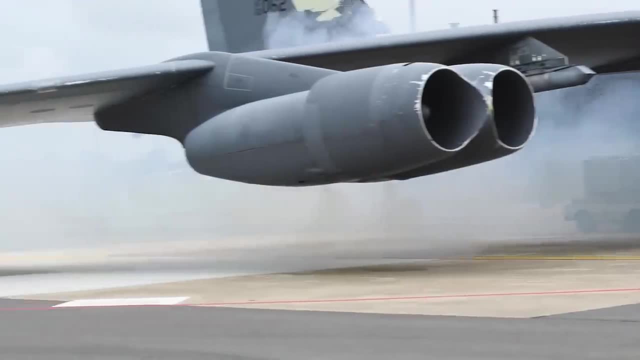 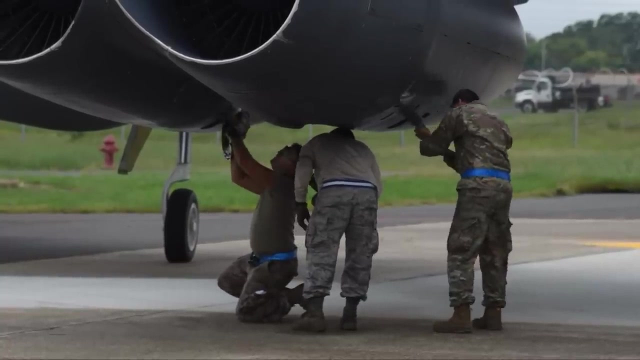 by an electric charge. The hot gas is expelled by the cartridge, then drive a smaller turbine which is connected to the drive shaft through a reduction gear allowing the smaller turbine to get the engines up to speed. Cartridge starters were popular in older military planes. 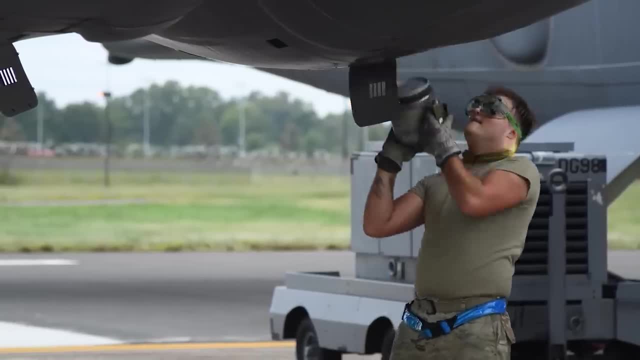 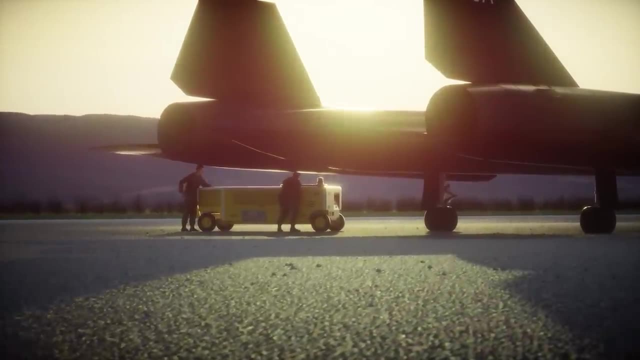 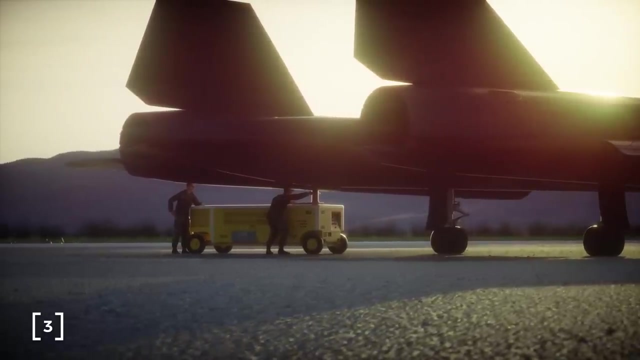 that may need to get in to the air on very short notice with limited ground support. Some planes like the SR71 had a direct drive starting cart which connected two massive V-8 engines directly to the J58 engine from underneath the nacelle to get the powerful jet engines. 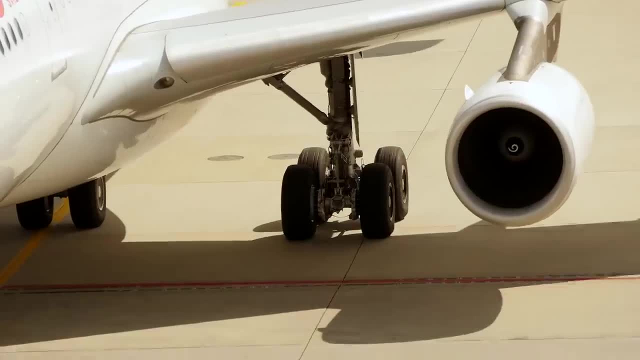 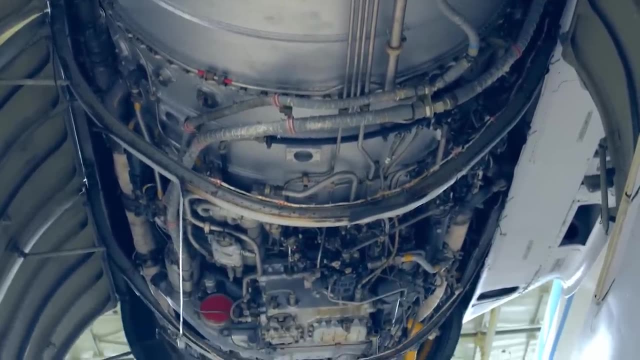 up to 4500 RPM. However, air starting is by far the most common method where pressurized air is fed into the turbine section directly to get the engine to power engine moving. This can be done with an external cart called a hover cart, which connects hoses. 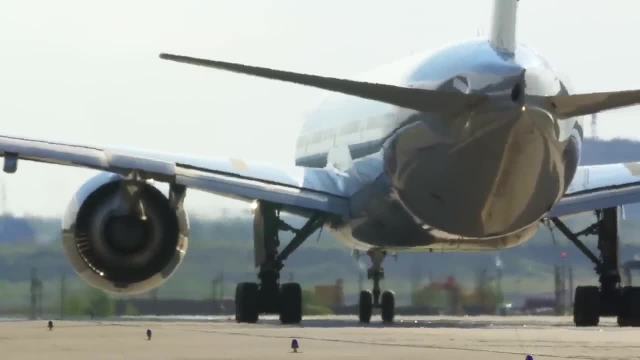 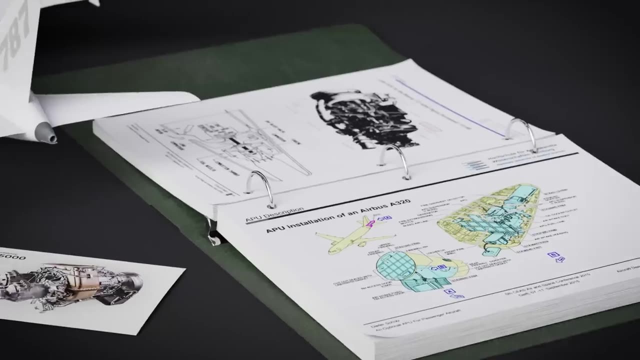 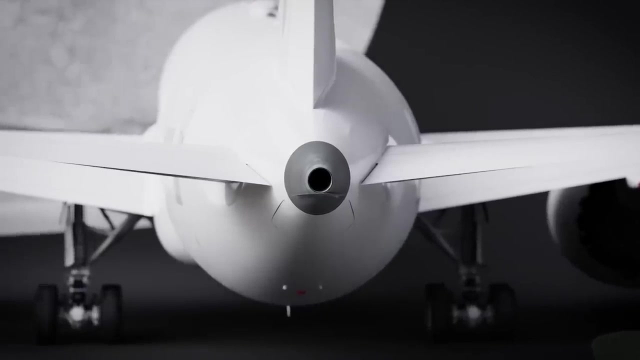 to the engine, But most commercial airliners are capable of generating their own pressurised air with an APU or auxiliary power unit. These are smaller turbine engines located at the tail of the aircraft that are small enough to get started with a battery and an. 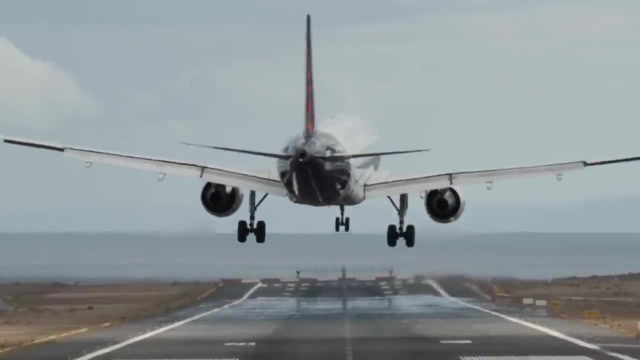 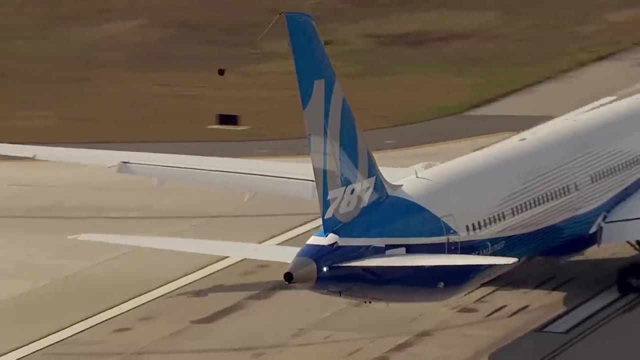 electric motor. Most people aren't even aware this mini turbine engine exists, but you can see the exhaust here on all modern commercial airliners. The 787's APU, like other planes, is started by a small battery, But from here the 787's 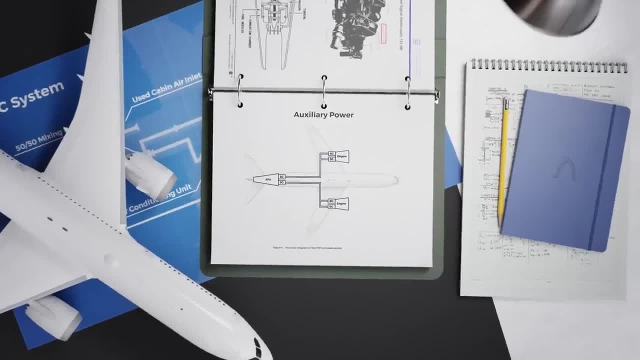 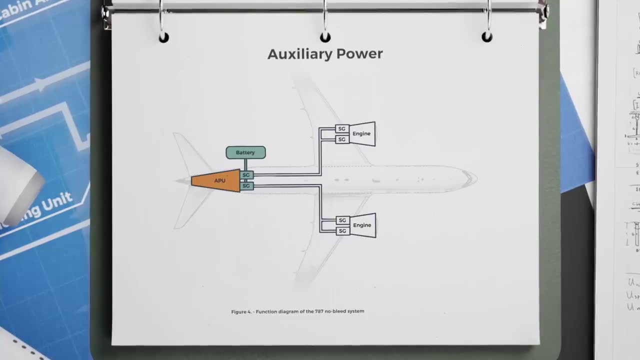 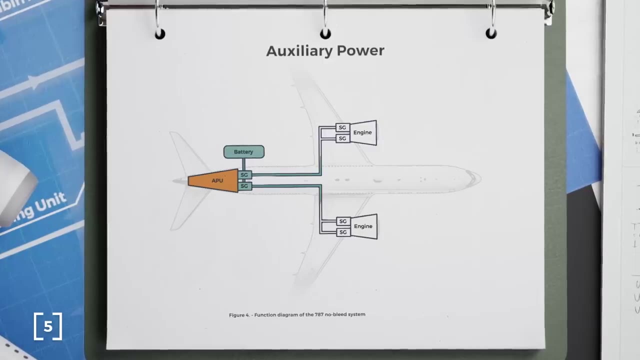 system architecture is very different. The 787's APU, like other planes, is started by a small battery, But from here the 787's system architecture is very different. The 787's APU does not provide pressurised air to the engines. It provides. 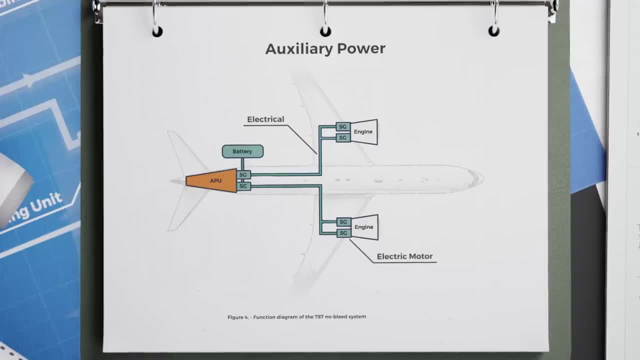 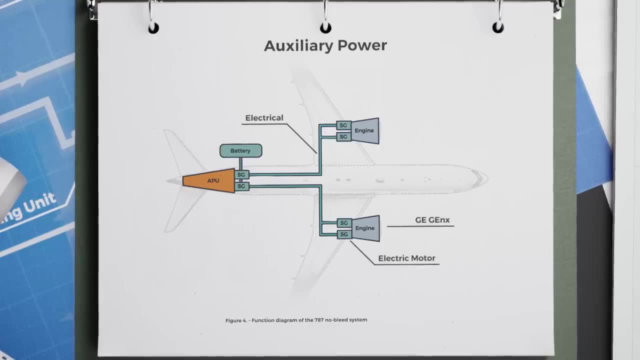 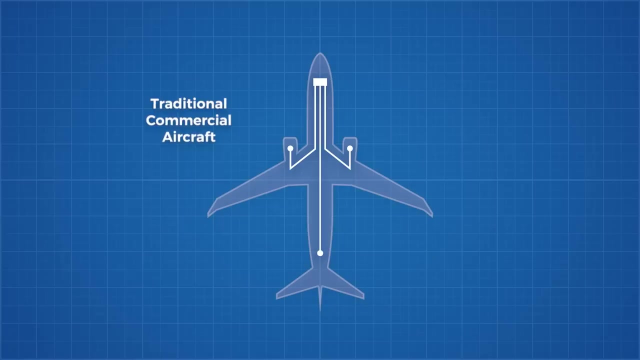 electric current to 2 electric motors attached to each engine which act like the starter motors on your car. However, these motors can act as generators to provide the 787 with unparalleled electric power. A traditional plane has one generator on each engine and one on the APU, But the 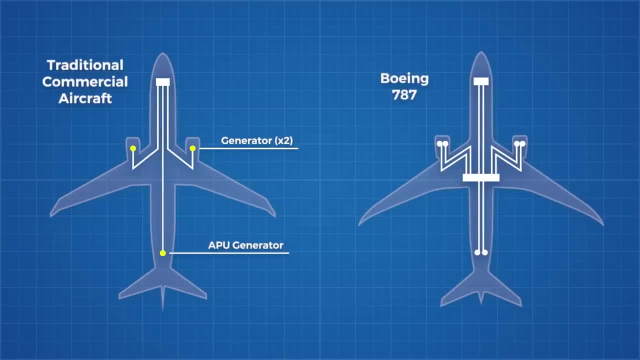 787 is anything but traditional. There are in total 6 generators on board, with two pairs on each engine providing the main power, Each capable of generating 250 kilowatts, With two more on the APU providing secondary power, Each capable of providing 225 kilowatts. 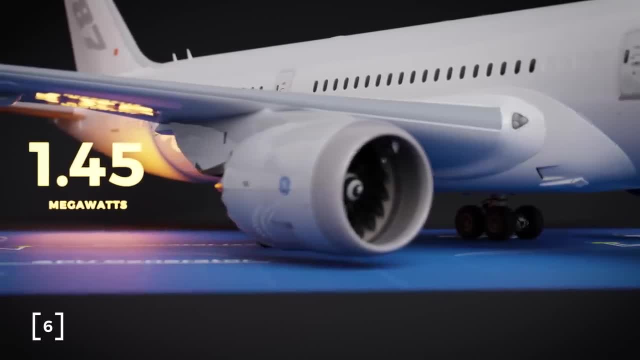 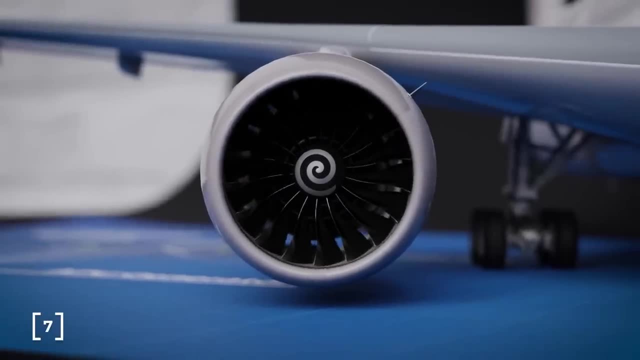 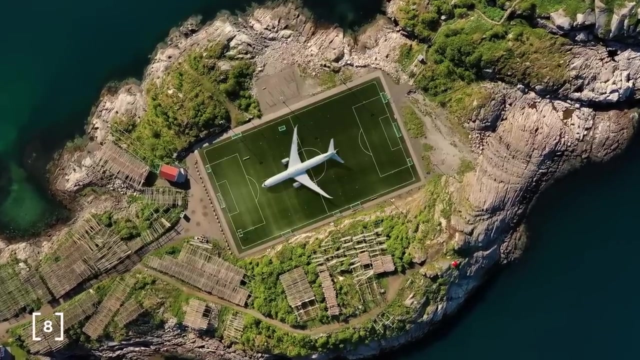 If all six of these generators were running at the same time, that would be 1.45 megawatts of power available to the 787. Four times more than a 777 is capable of producing. To put that into perspective, this is a 787 on a football field. If we needed to generate 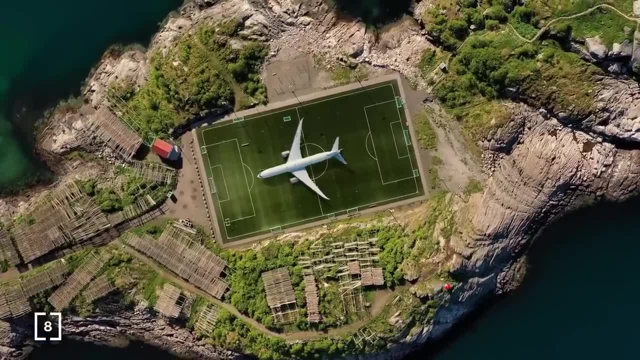 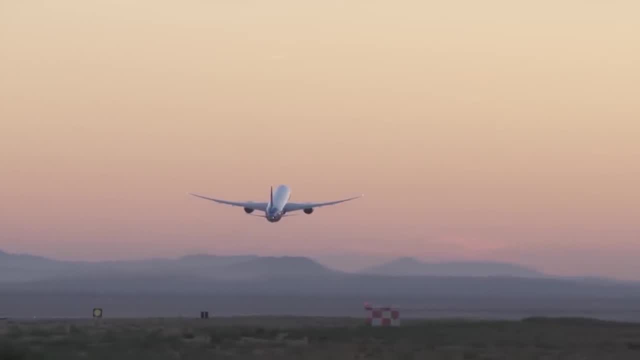 that electricity with solar panels. in the middle of the day, we would need to cover about 10 football fields with solar panels. This is a lot of power. so why did the 787 need that much power and where is it all going? 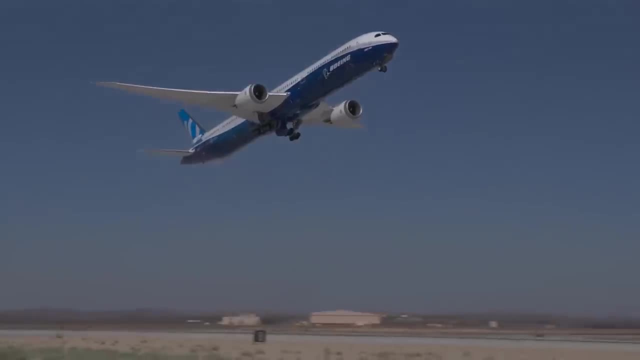 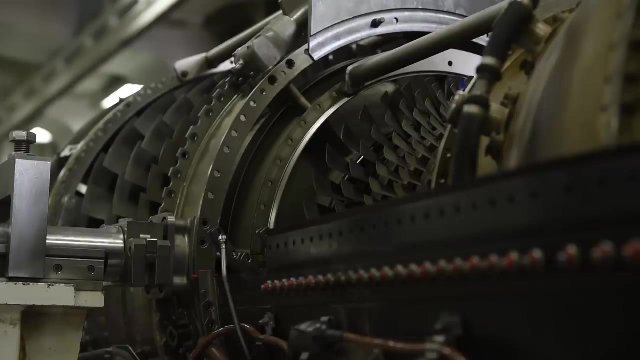 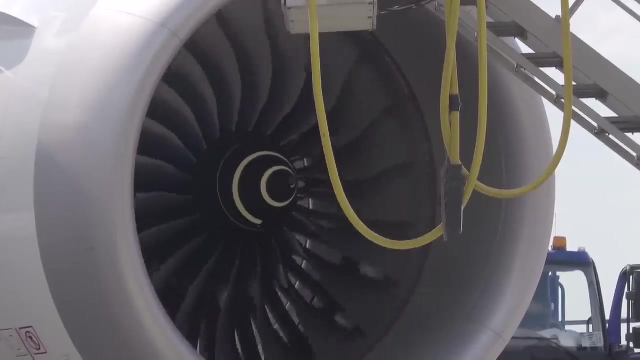 The 787 uses a no bleed air architecture. Traditionally, many aircraft systems are powered by hot compressors. The APU normally provides hot air to the engines to get them started and then, once the main engines are started, hot compressed air bled from the compressor section. drives several 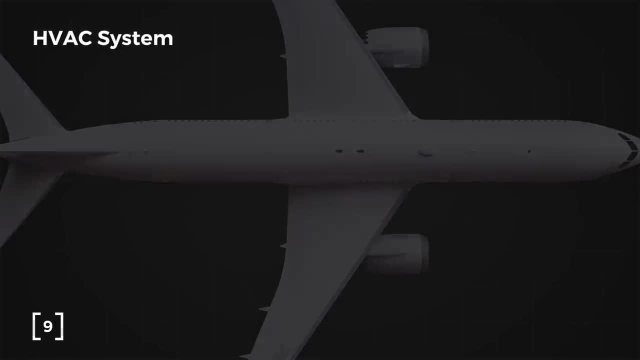 important systems. Normally, air conditioning and cabin pressurisation is handled by the bleed air system. The bleed air would be drawn from the engine at a temperature upwards of 230 degrees celsius. This obviously would quickly reduce the pressure on the engine. The bleed air would be drawn. 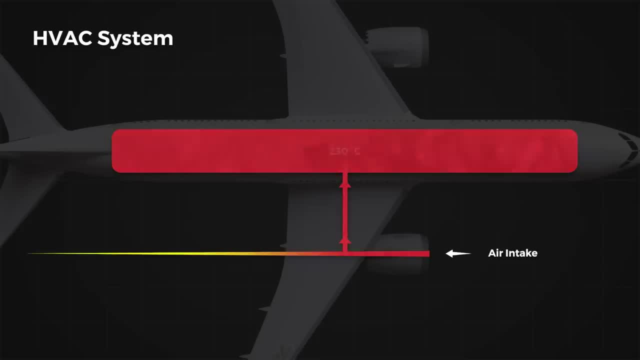 from the engine at a temperature upwards of 230 degrees celsius. This obviously would quickly turn the cabin into an oven, so the air would first run through a complicated air conditioning and pressurisation system, where some of the air is cooled using a heat exchanger which 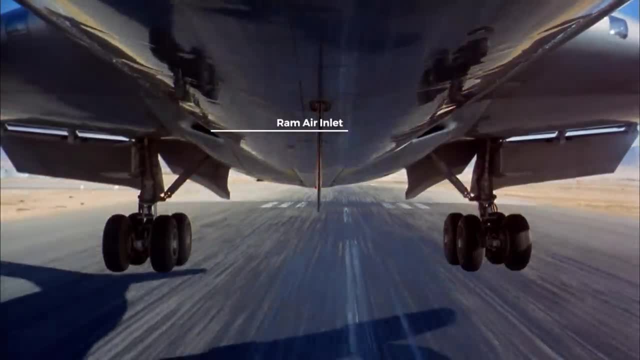 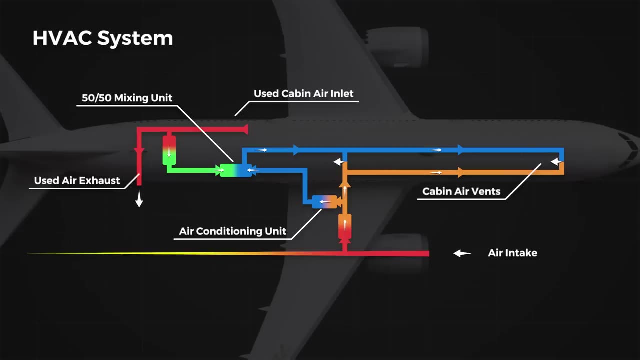 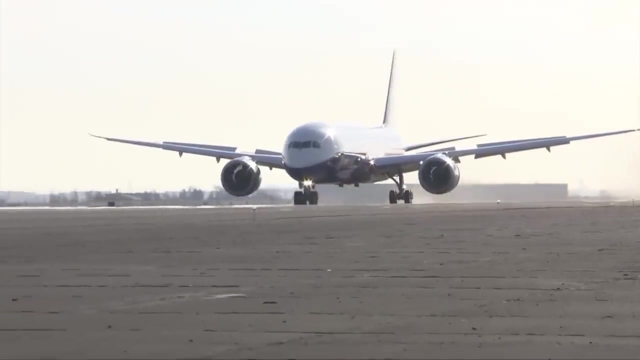 uses outside air from a surface mounted intake called ram intakes to remove heat from the engine bleed air until it is a suitable temperature to be distributed through the cabin. So we are doing work to remove energy from this valuable bleed air from the engine. This 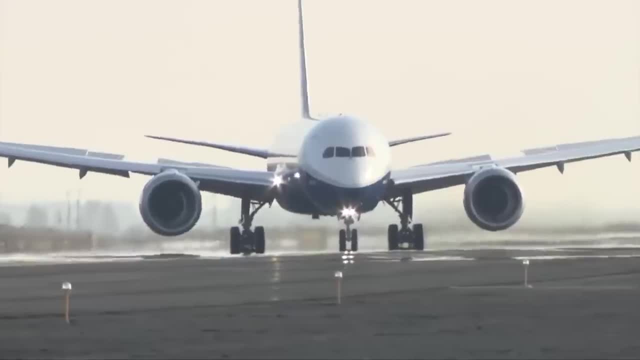 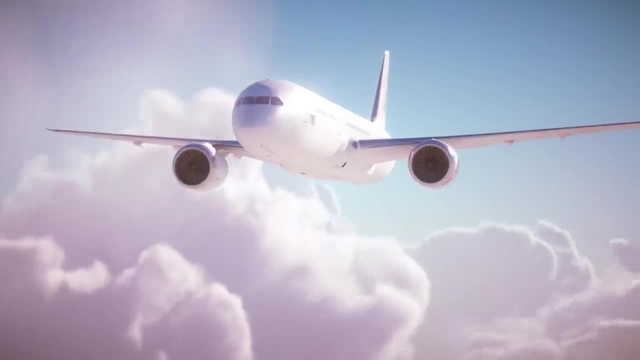 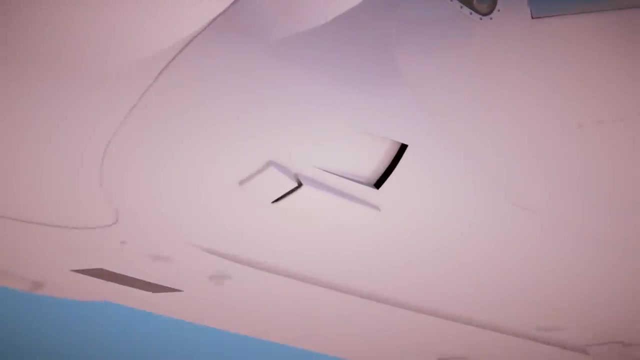 is obviously rather inefficient and all that ducting is heavy, And this is why the 787 does not use this system. Its cabin pressurisation is handled entirely electrically. We now have two inlets: The ram air inlet and the cabin air compressor inlet. 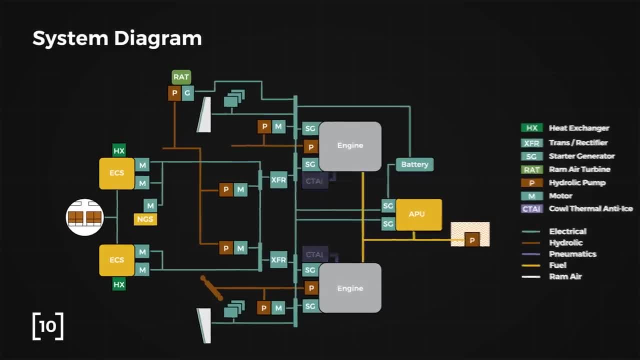 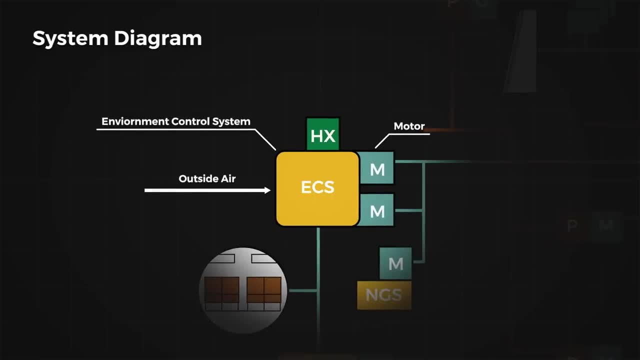 The cabin air compressor leads to. you guessed it: the cabin air compressor, An electrically driven device that compresses the air for the passenger cabin. This compression process heats the air up too much for direct use into the cabin, so it does require some cooling. 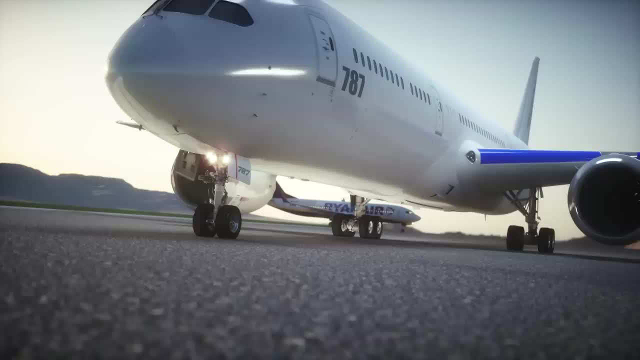 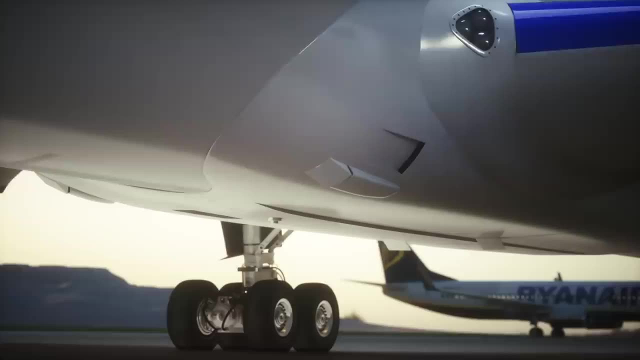 using a heat exchanger cooled by the ram air inlet. You can see this little door open while the plane is on the ground, and it serves to protect the inlet from foreign objects entering it. Another energy intensive process that has been handed over to the electric motors is 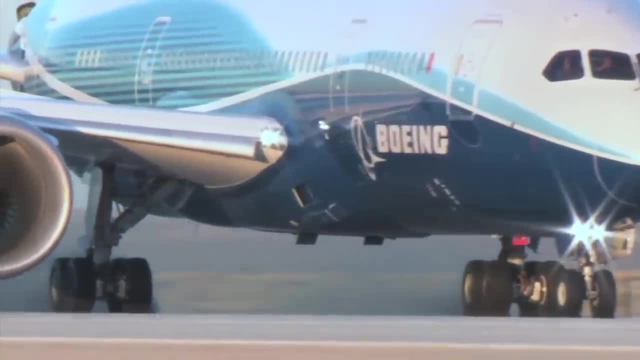 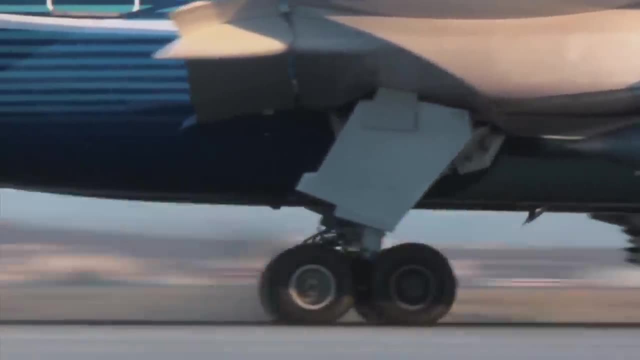 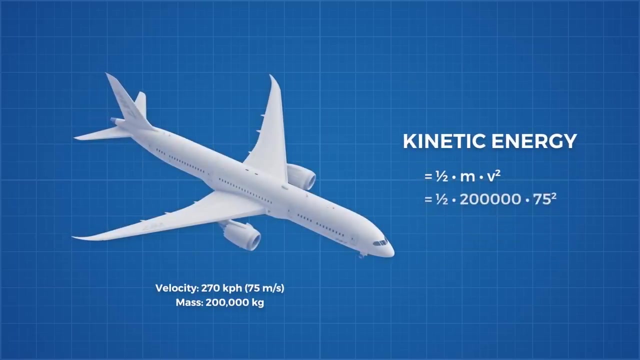 the braking system. As you can imagine, the energy required to slow down a 200 ton plane travelling at 270 kilometres per hour is not small. Calculating the energy required is pretty trivial. We just need to calculate the kinetic energy of the object, which we can do with this equation and that gives us a kinetic 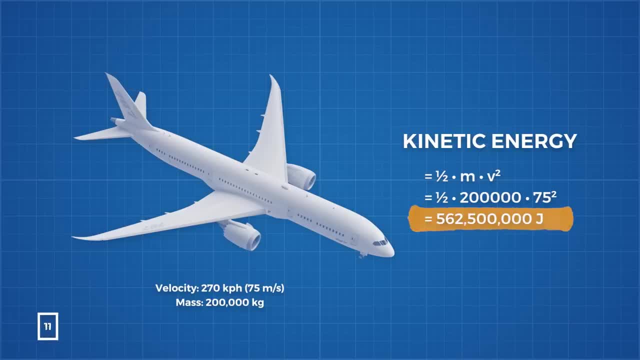 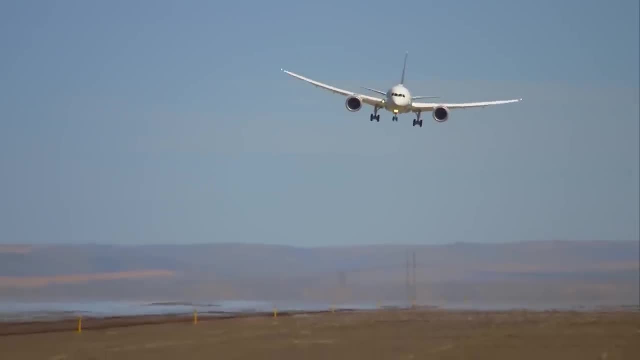 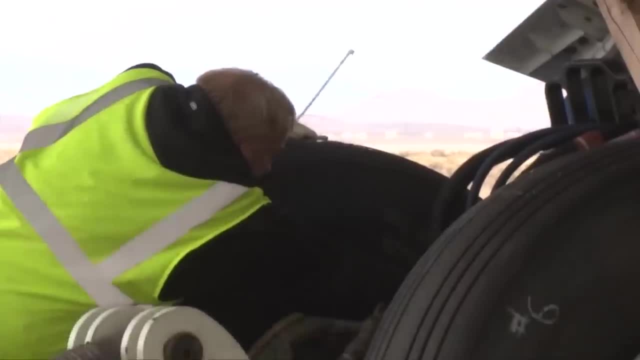 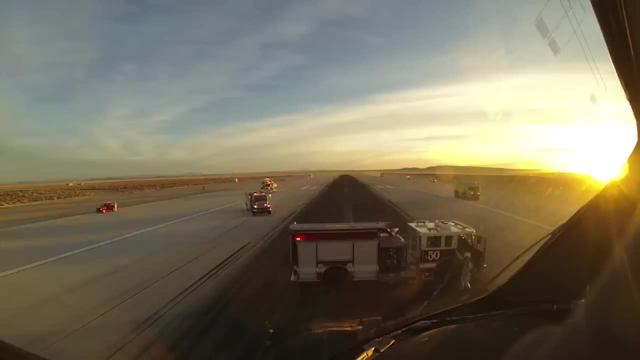 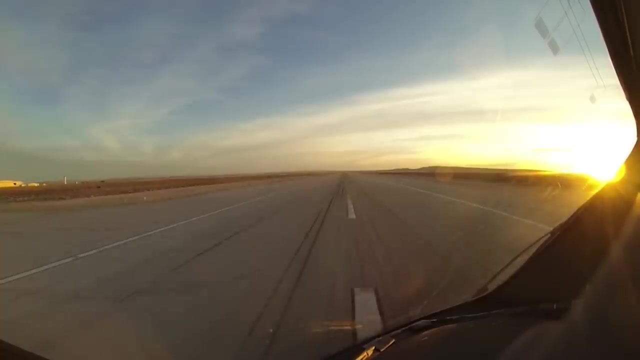 So the brakes need to convert a lot of kinetic energy into another form of energy: heat energy. You can really see this in effect during a plane's most extreme brake test, an aborted landing test. Here the plane is flying at full load, including the weight of the fuel. 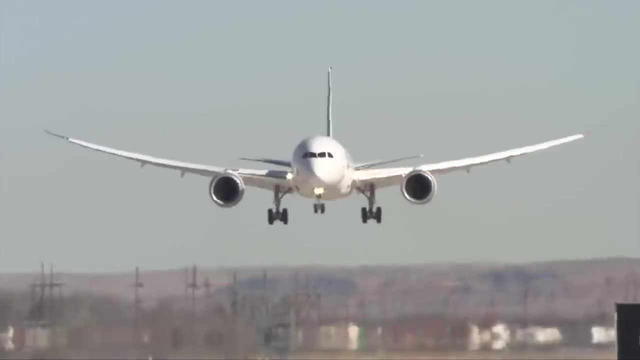 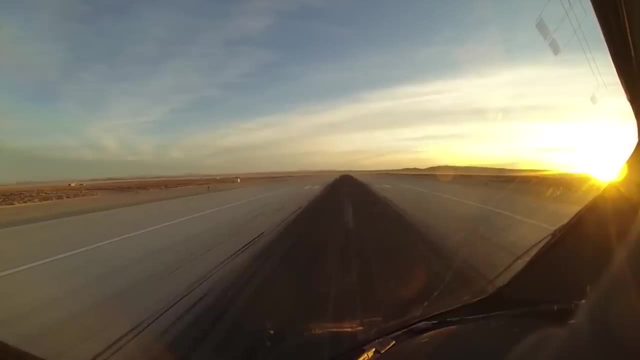 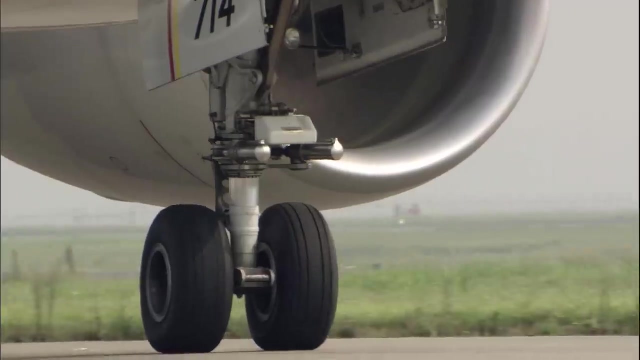 and has to abort at its V1 speed, the absolute maximum speed a plane can abort a landing at. From that point, the plane has to take off. When the plane comes to a full stop, the brakes are glowing red hot. Typically, the braking mechanism of planes is driven by hydraulics with a hydraulic 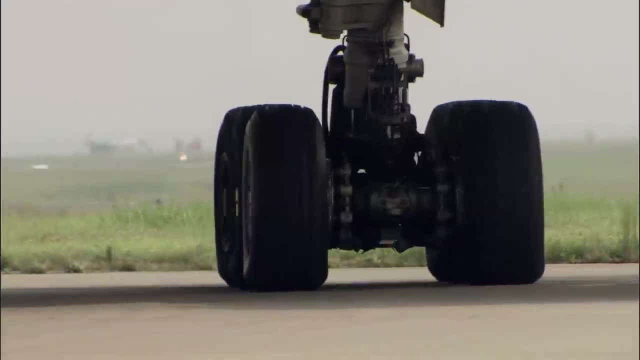 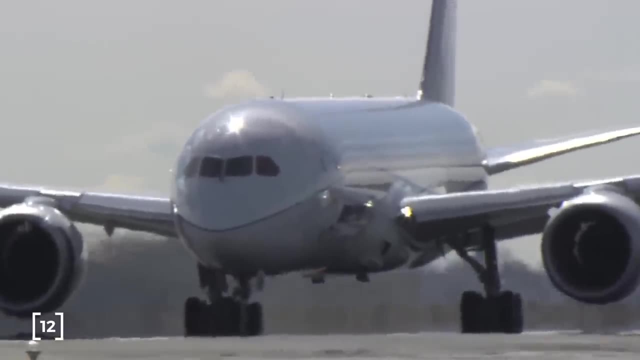 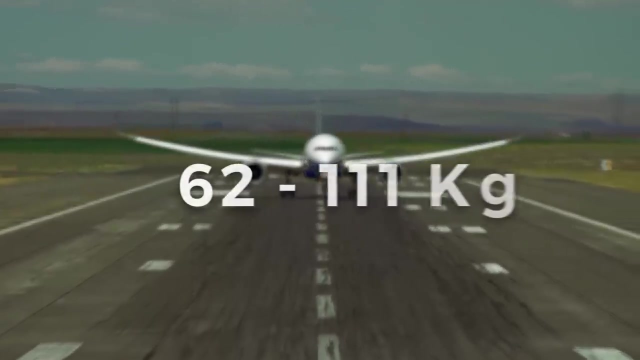 pist enforcing the brake pads against the wheel to slow down the plane. The 787 removed this bulky hydraulic system and traded it in for brakes actuated by electric motors. Each of the 8 landing gear wheels feature one of these units and together they helped. 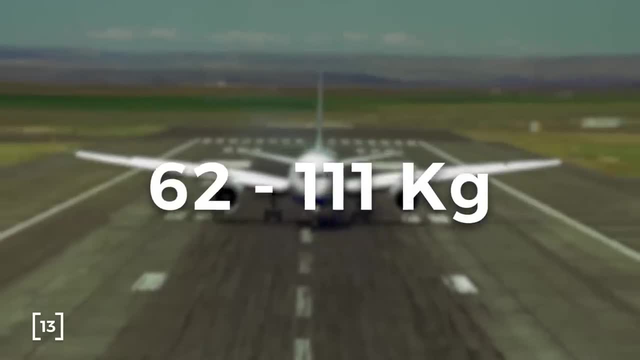 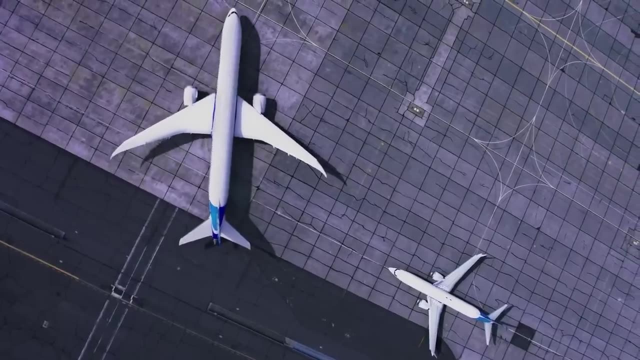 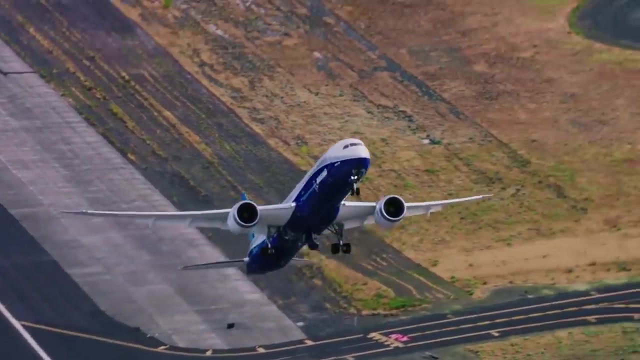 eliminate between 62 to 111 kilograms of weight from the 787, while also being drastically easier to maintain and install. The 787 does have a hydraulic system, however, but it has eliminated two large bleed air driven hydraulic pumps that are normally used to meet peak demand during take off and landing. 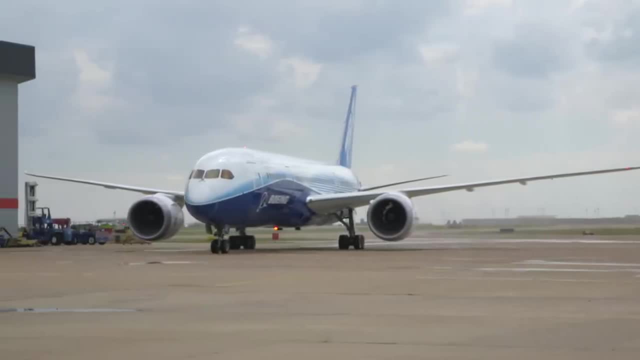 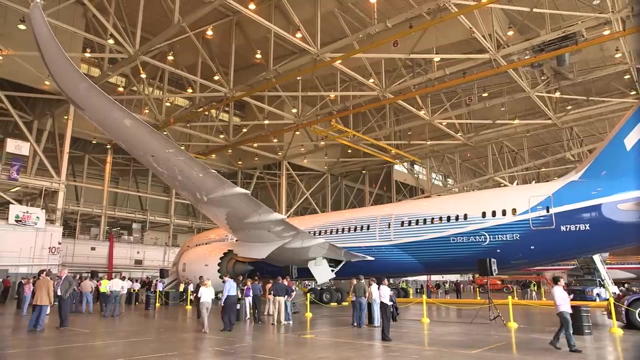 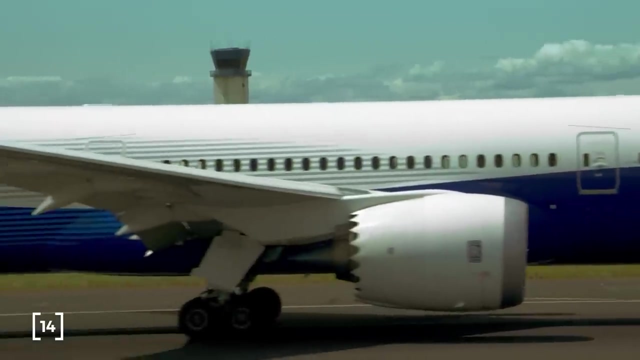 where landing gear actuation and deployment of high lift devices like slats and flaps would overload the other pumps that power the hydraulic system. The 787 had the added electric power needed to rid itself of these bleed air powered pumps and replaced them with more efficient electrically driven pumps. 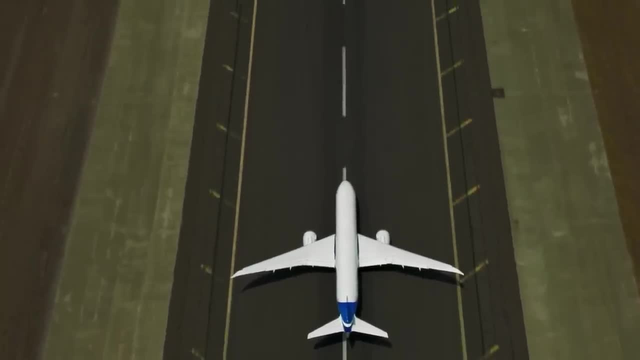 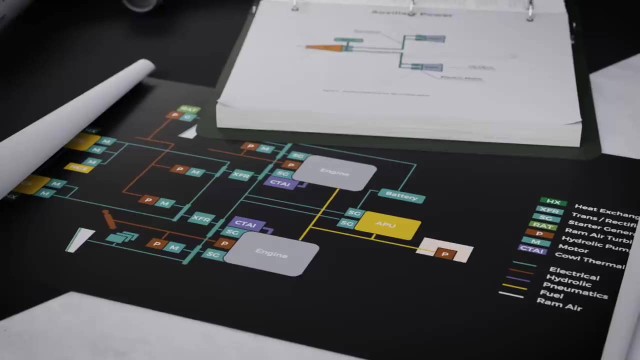 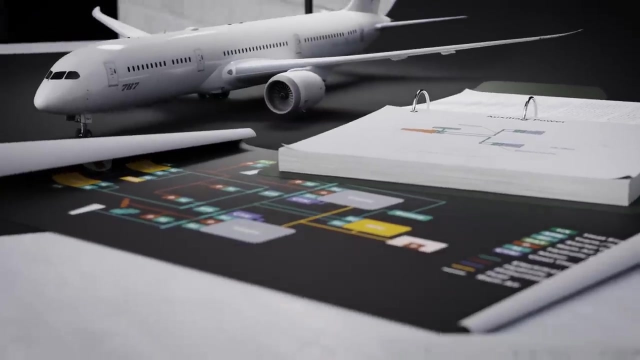 To boot. the 787 is able to generate higher hydraulic pressures that allow it to use smaller hydraulic components, which saves both weight and space. So that covers most of the system architecture, but we haven't even touched on the revolutionary engine's design. 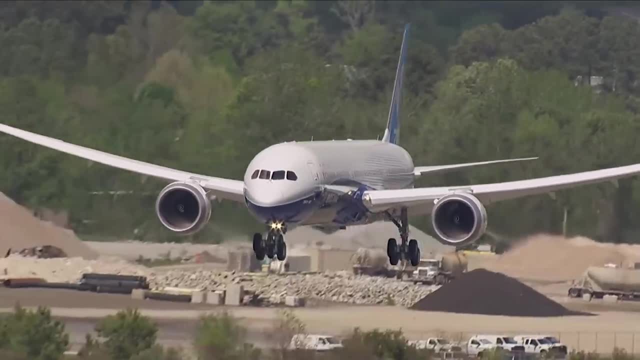 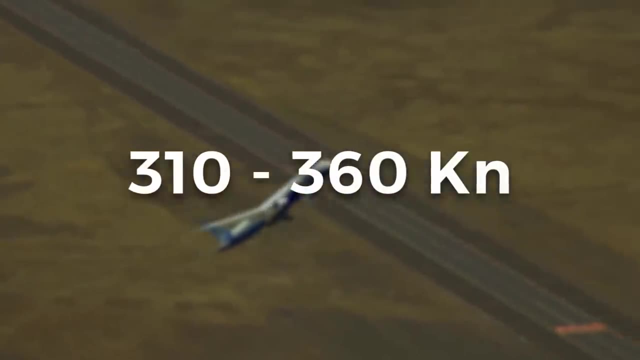 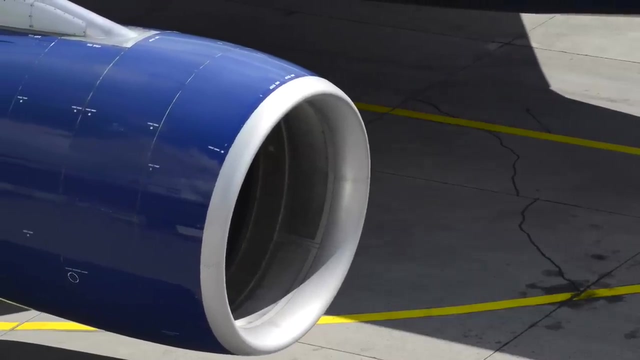 The Dreamliner is most commonly fitted with two General Electric GE-NX engines, each capable of producing between 310 kilonewtons and 360 kilonewtons of thrust- About the same thrust that General Electric's previous generation engines, the CF-6 equipped. 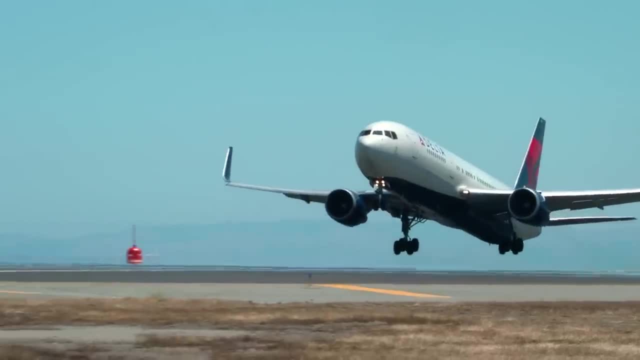 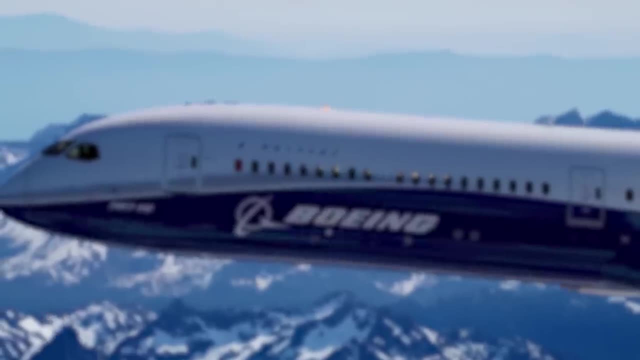 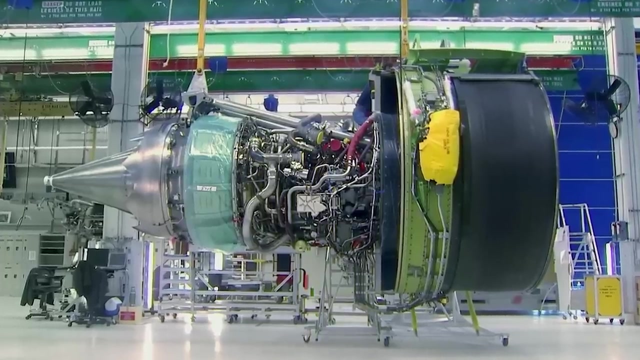 the 767, were capable of producing, but the GE-NX produces this thrust while consuming 15% less fuel. That's an incredible leap in technology. The GE-NX achieves this primarily through two major design features that were not possible with older engines. 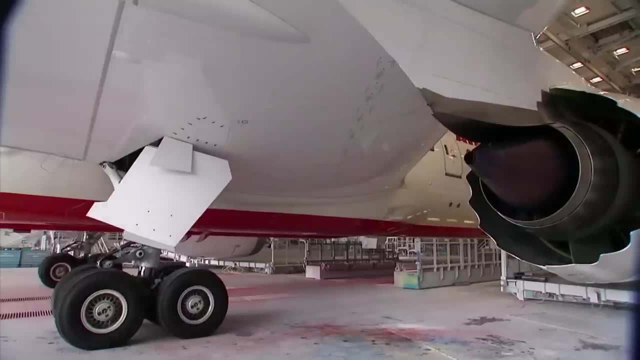 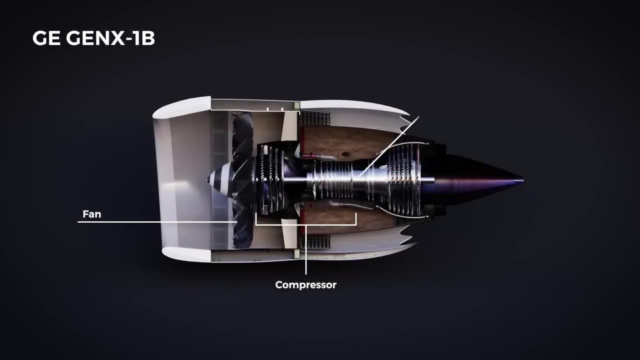 The first is a gigantic bypass duct that surrounds the main engine. The primary components of modern day jet engines are the fan, a compressor, a combustor, a turbine and a nozzle. The ultimate goal of a jet engine is to draw in air and pressurise it. 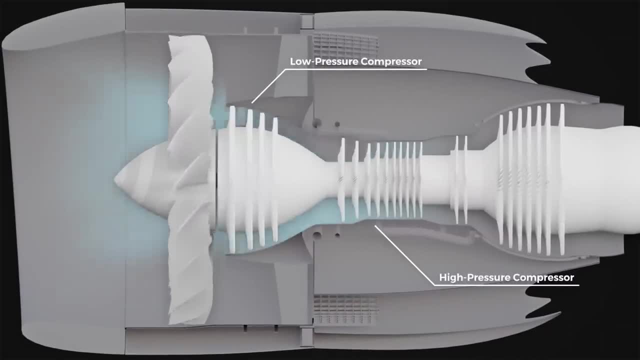 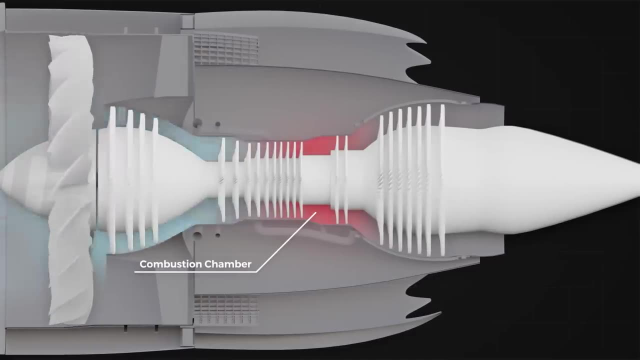 This means that the engine will be able to produce more fuel than the engine itself. pressurise it as much as possible, which increases the energy potential of the air, before mixing it with fuel and igniting it, causing a rapid expansion and acceleration of air. 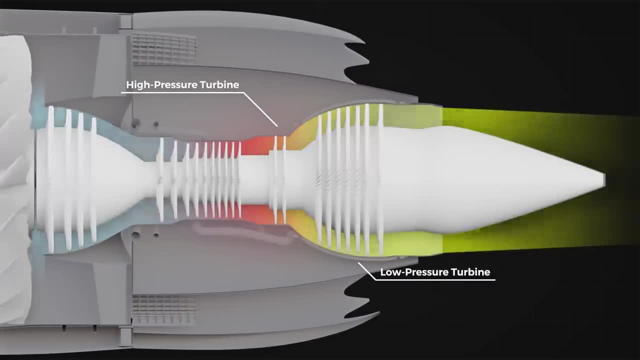 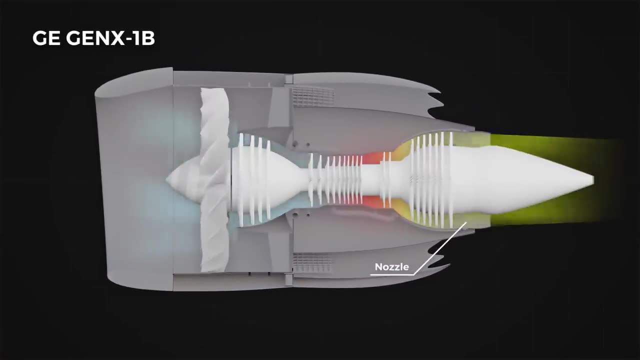 The work done by the compressor is then recovered in the turbine section, which powers both the compressor and the fan. Finally, the air with its remaining kinetic energy travels through the nozzle, where it is accelerated more and sent out the back of the engine to provide thrust. 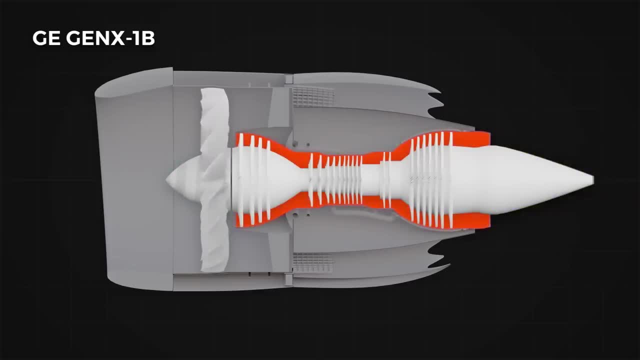 The engine core. this part of the engine is what powers the engine. Yet most of the air that travels through the GE-NX bypasses this section completely, only passing through the fan and through this bypass duct, and this is one of the reasons the engine 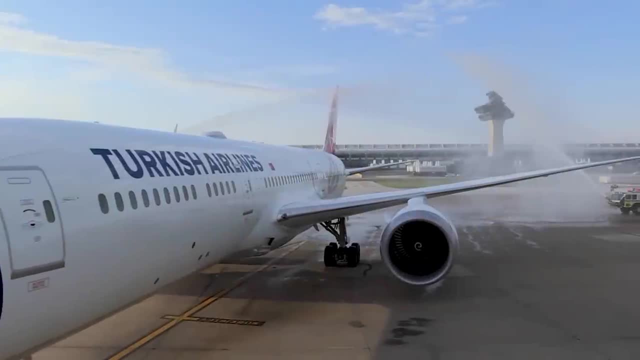 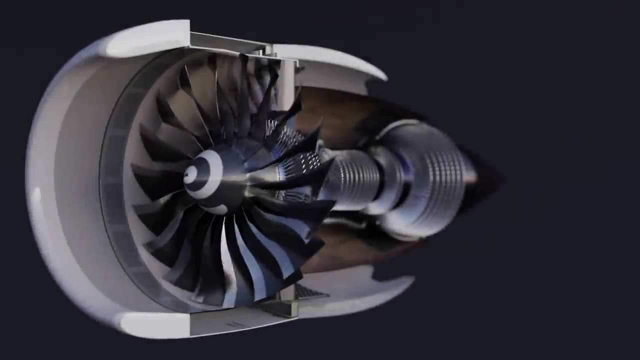 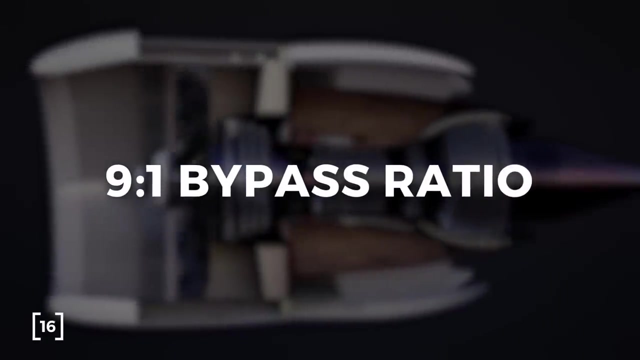 is so incredibly efficient. Bypass ratios have continually increased over the years, which is one of the reasons engines keep getting bigger. The GE-NX engine has a bypass ratio of 9 to 1, meaning for every kilogram of air that passes through the engine core, 9 kilograms flow through the bypass duct. 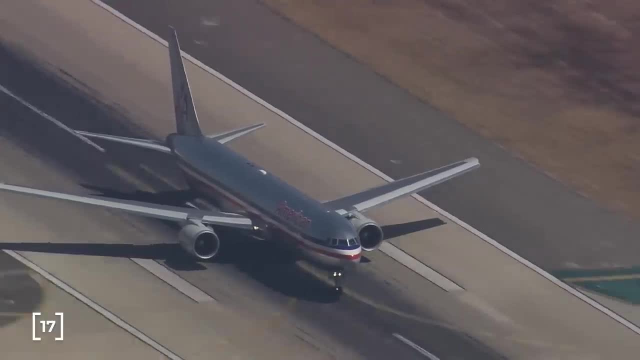 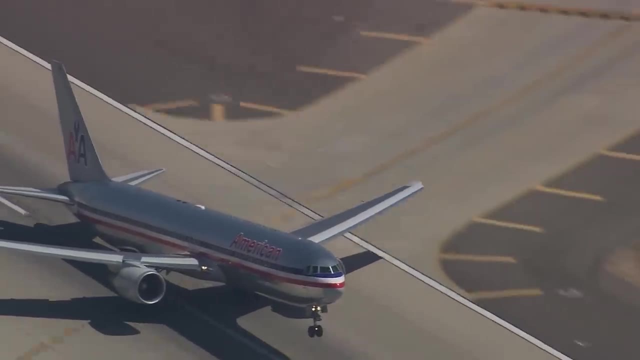 This is extremely high. The engine the GE-NX replaced only had a bypass of 5.7, which during its time, was itself a very high bypass ratio. While the core takes a small volume of air and accelerates it rapidly, the fan takes. 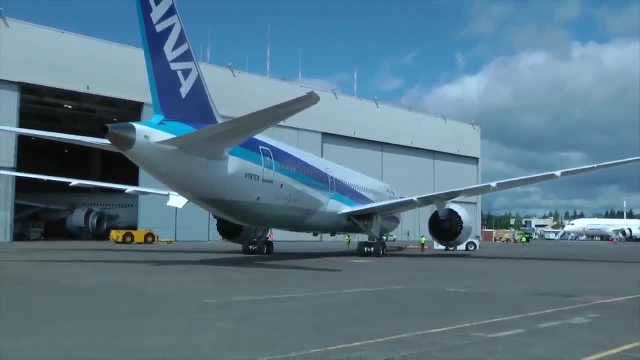 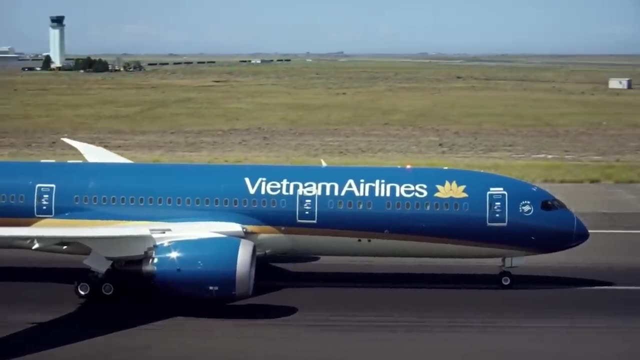 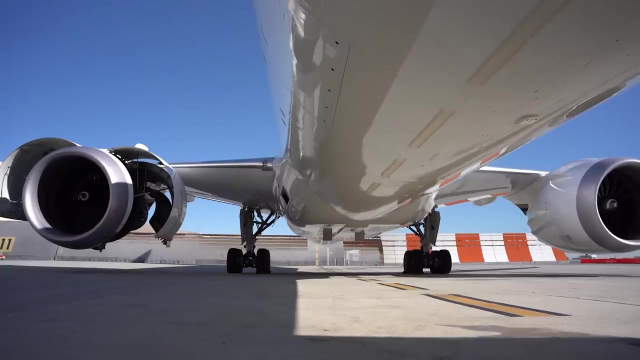 a massive volume of air And accelerates it just a little, while not requiring it to be mixed with fuel and ignited. This drastically increases the fuel efficiency of the plane. The fan essentially acts like a gigantic propeller. The industry has been aiming for larger and larger bypass ratios for decades, but there 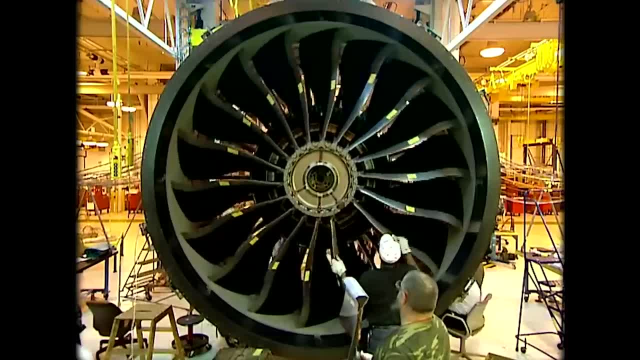 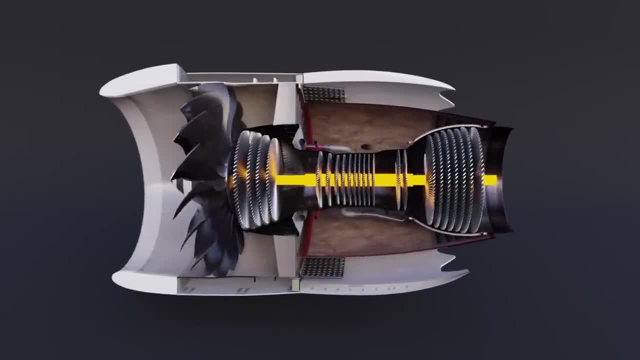 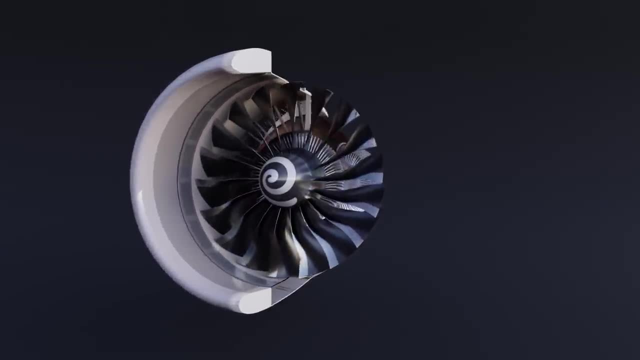 are a couple of limiting factors that make it difficult to increase the size of the fan blades. The compressor and fan are driven by the same shaft, Meaning they rotate at the same speed, But because the fan is so much larger than the compressor and turbine blades, the fan 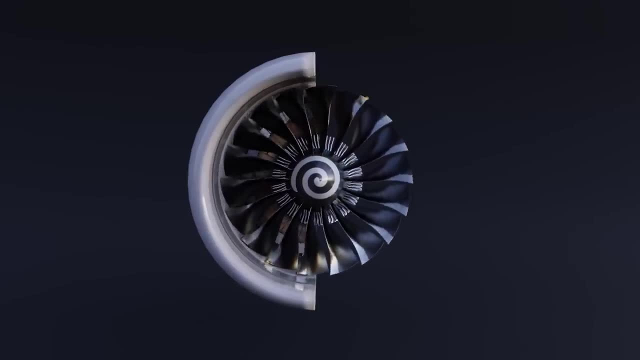 experiences much higher centrifugal forces, And if the fan blades grow too long, their tips could even break the speed of sound, leading to shockwaves and a massive increase in drag. The first problem we need to address is how to handle those centrifugal forces. 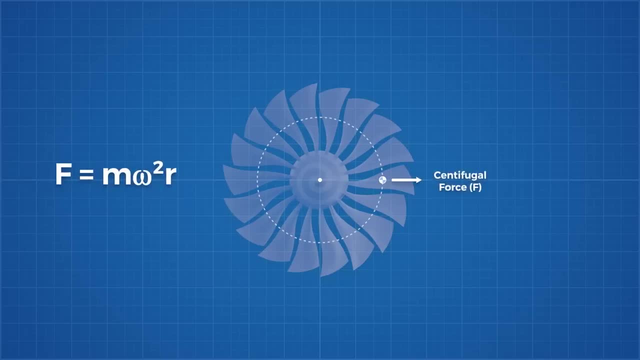 The magnitude of the centrifugal force can be found using this equation, where m is the mass, w is the angular velocity and r is the distance from the centre of rotation. So our force will increase with the weight of the blade, the speed of its rotation and 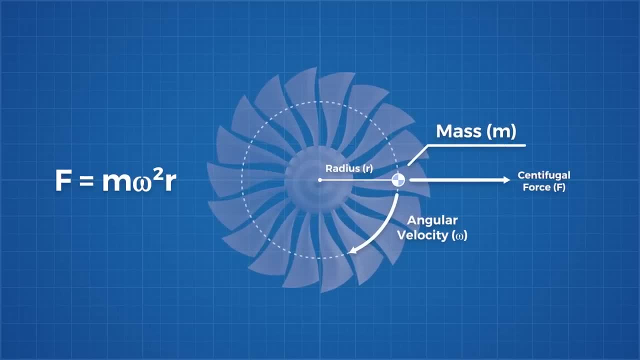 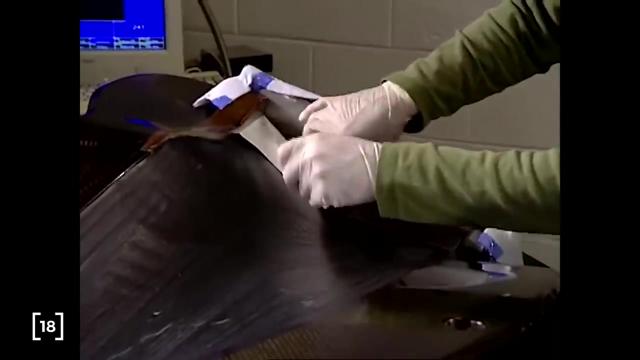 its diameter. We want to increase our diameter, to increase our bypass ratio, So we need to figure out ways to either decrease our weight or decrease our rotational speed. The GENX achieved the first requirement by using lightweight carbon fibres- Carbon fibre fan blades. 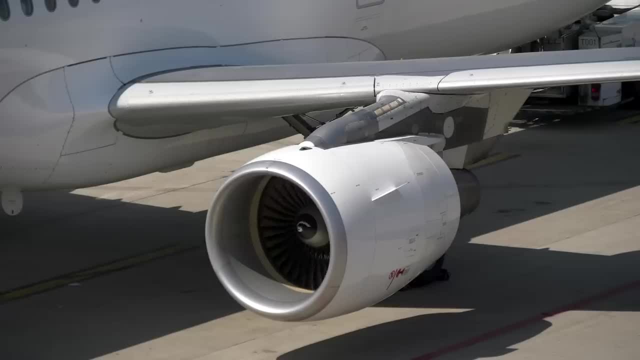 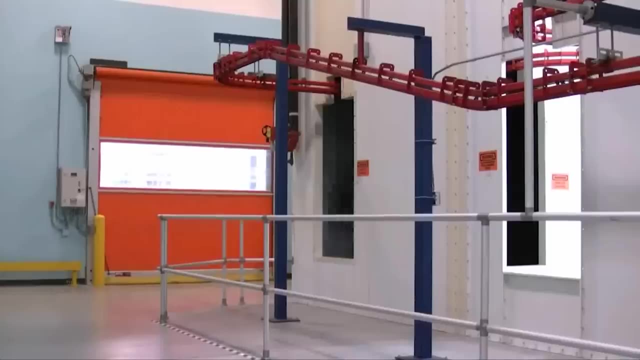 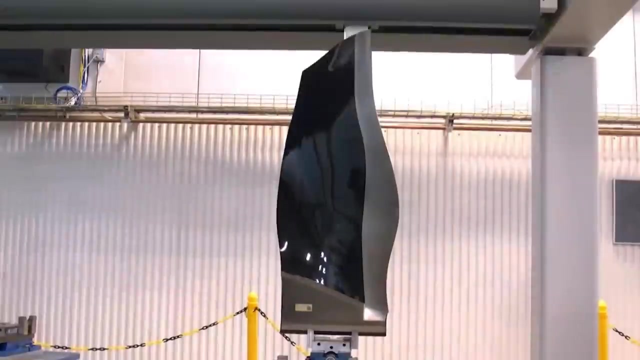 Older fan blades were constructed from titanium, Titanium being used for its excellent strength to weight ratio, But carbon fibre blades have an even higher strength to weight ratio, while also being much stiffer than titanium, Allowing the carbon fibre composite blades to be longer and thinner than their titanium. 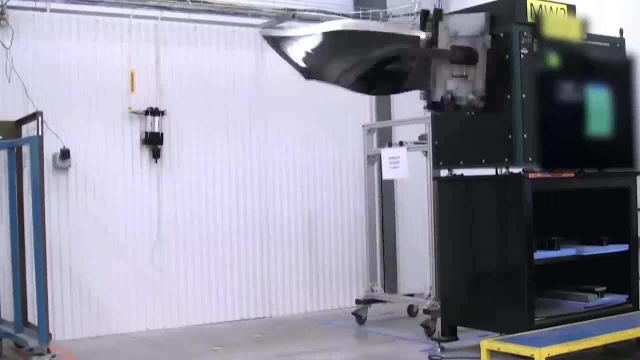 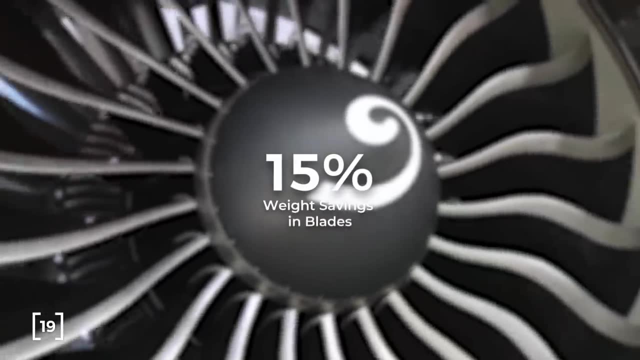 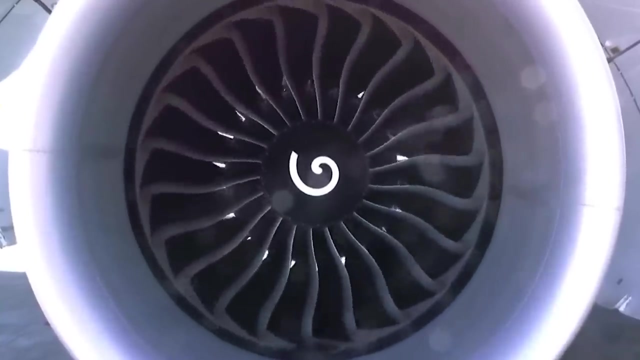 counterparts. This form factor even allowed General Electric to reduce the blade count from 22 to 18.. In all, this resulted in a 15% weight savings in the blades, allowing them to spin faster without worry of damage. However, composites do have one huge drawback. 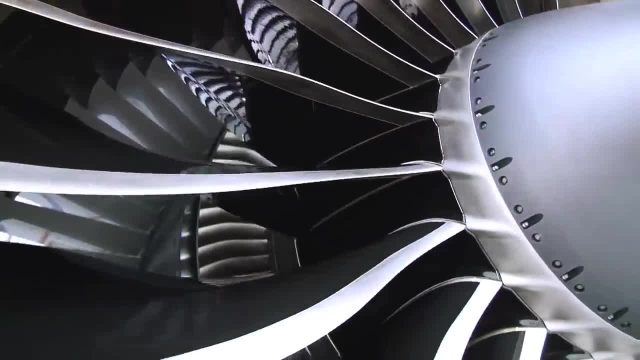 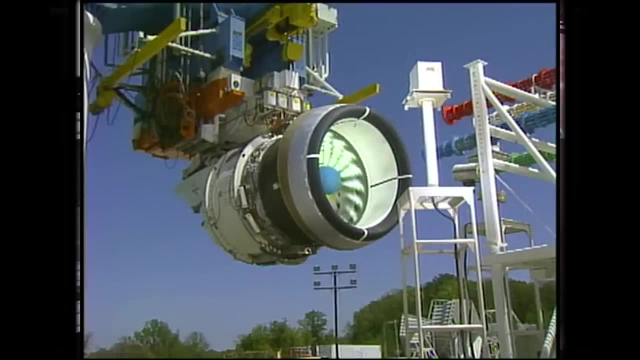 Their impact resistance. One of the tests engine need to pass to reach certification is the chicken gun test which, as you may have guessed, involves yeeting a dead bird into the engine and seeing how it holds up. The fan blades are the first part of the engine. 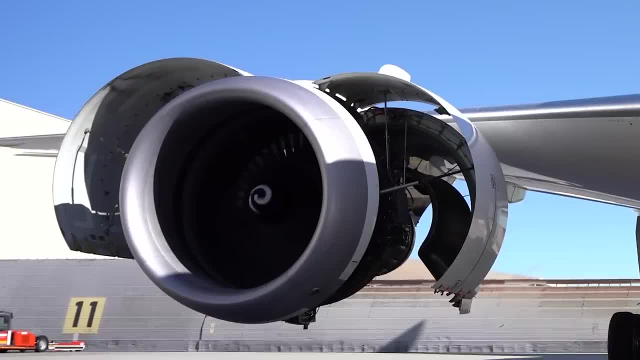 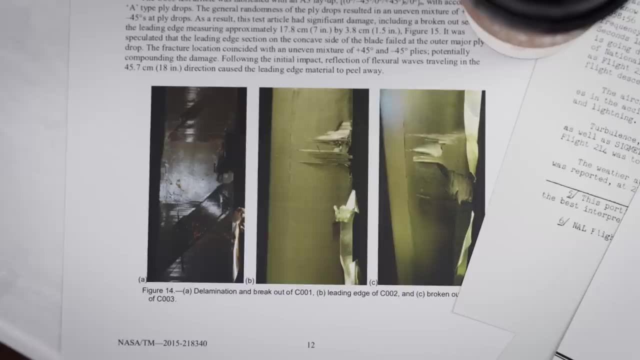 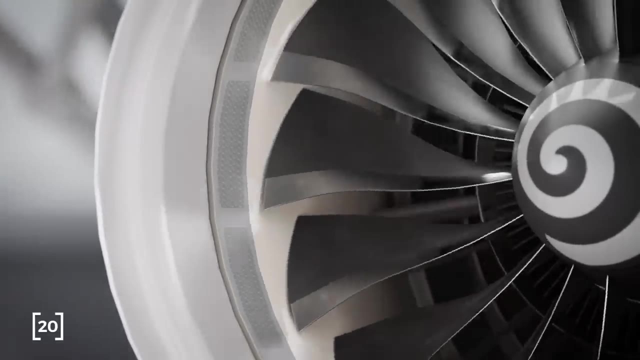 Any foreign object will encounter and thus need to be capable of withstanding the impact. Early development of composite fan blades by NASA and GE showed that composite blades by themselves simply were not up to the task. To solve the issue, the leading edge of the blades are reinforced with titanium. 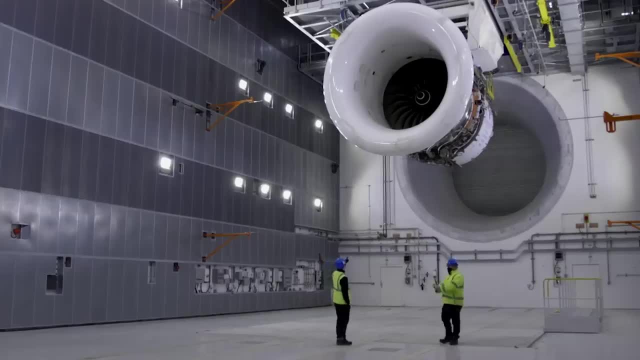 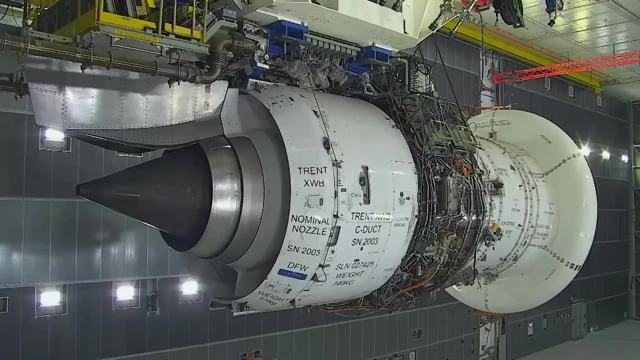 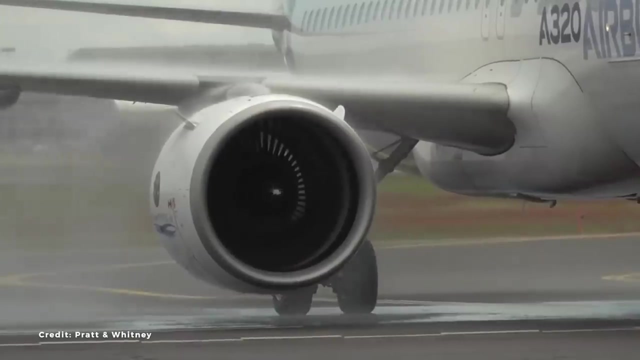 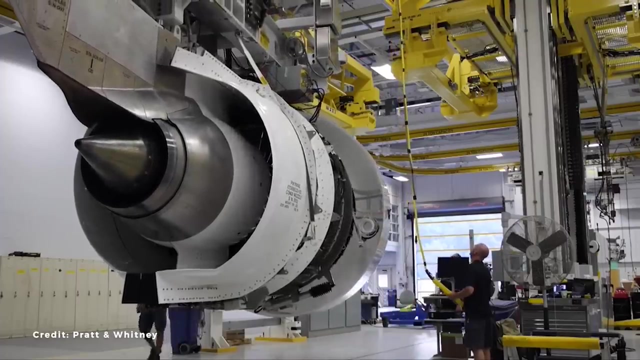 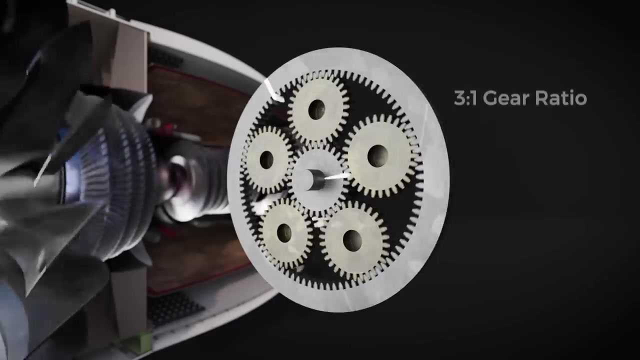 Bypass ratios are likely to continue growing as our technologies develop. Speed reduction gears between the main drive shaft and the fan may allow engine manoeuvrage. The They included a planetary gear between the main drive shaft and the turbofan drive shaft, which applied a 3 to 1 reduction in speed, allowing the turbofan to spin at a lower 4-5,000. 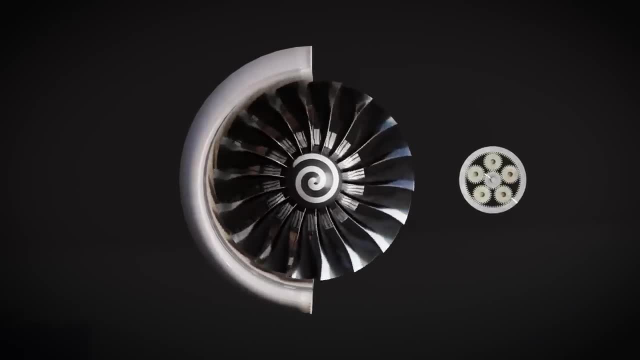 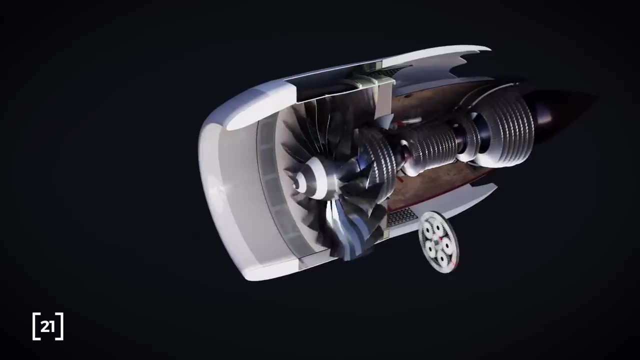 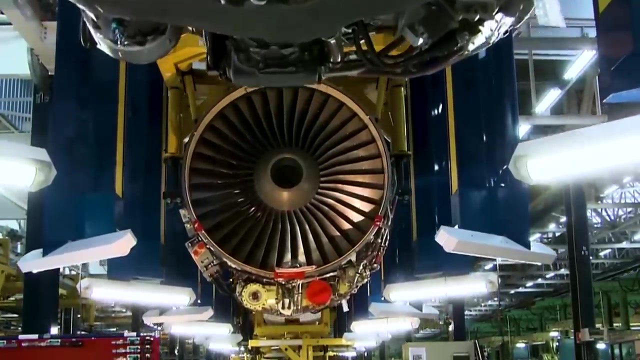 rpm. This enabled the fan to grow in diameter, as the forces the larger blades had to endure were drastically reduced with a lower speed, Giving the engine a record breaking 12.5 to 1 bypass ratio. The design of General Electric was considered for their new LEAP engine, currently in use. 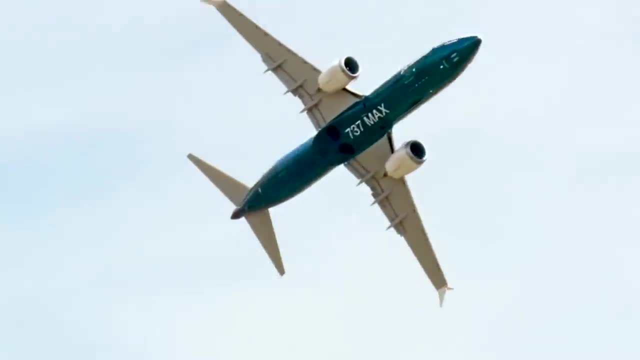 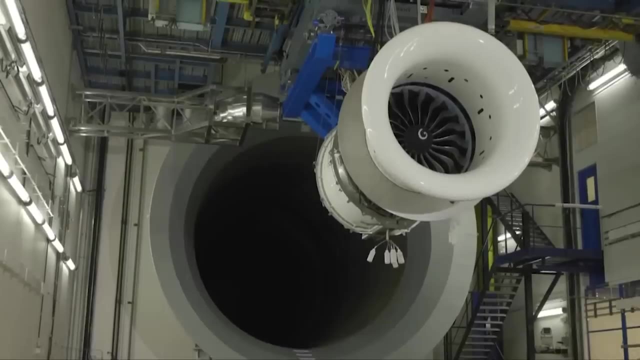 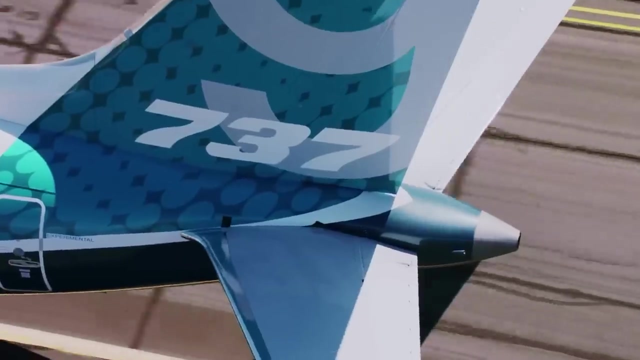 by the 737 MAX, but problems with weight and maintenance of the planetary gearbox deterred them. That hesitance may have been justified as the engines have had a turbulent operation history, with several groundings and engine removals, although these issues were not directly. 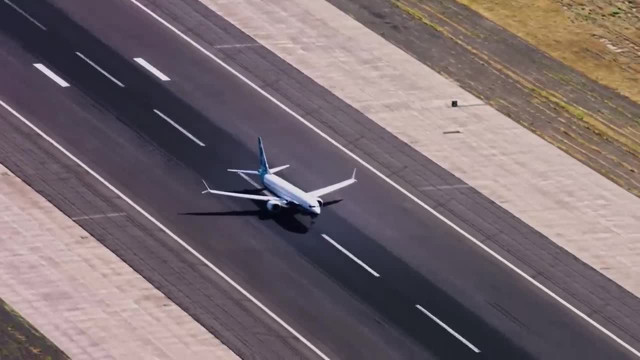 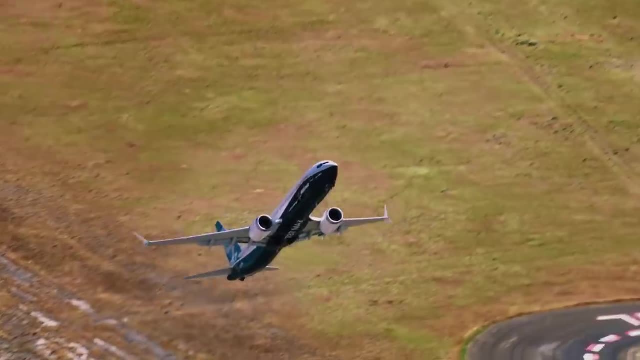 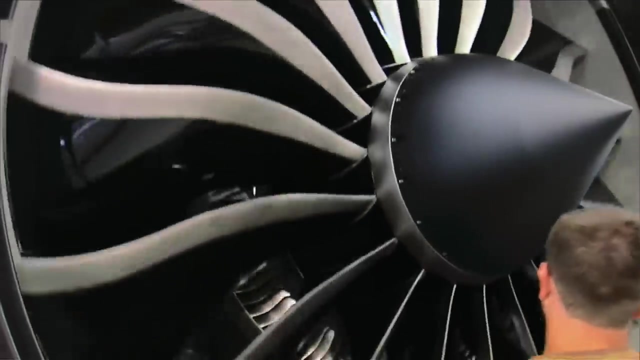 a result of the planetary gears. However, as the technology improves, we may see more of these geared designs being used to drive even greater fuel savings. The next designed feature that helps the GE-NX to reduce fuel consumption is the extremely high compression ratio. 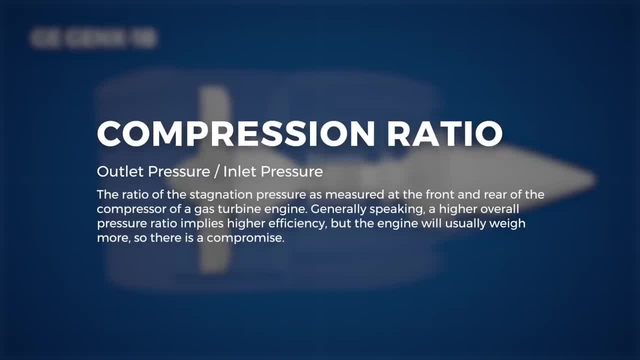 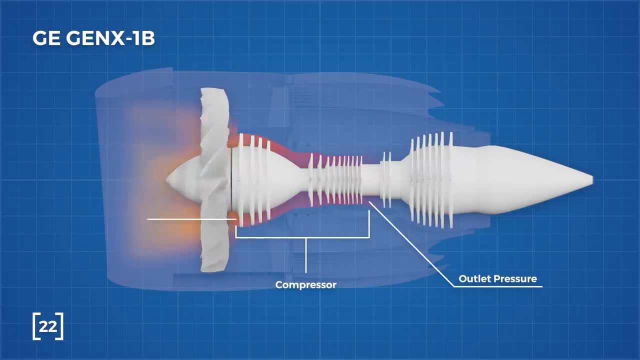 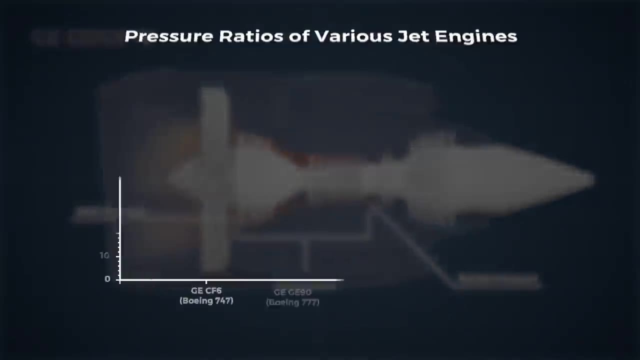 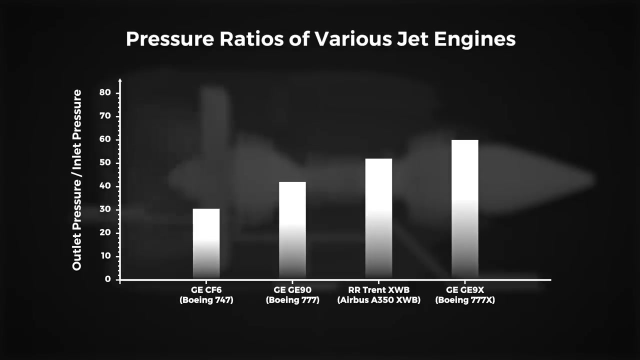 Compression ratio achieved through the engines compressor section. Compression ratio is the ratio found by dividing the pressure at the exit of the compressor section by the pressure at the inlet. This one variable has huge implications for a planes fuel efficiency and just as we can see a clear upwards trend for bypass ratios over time, the same can be seen for pressure. 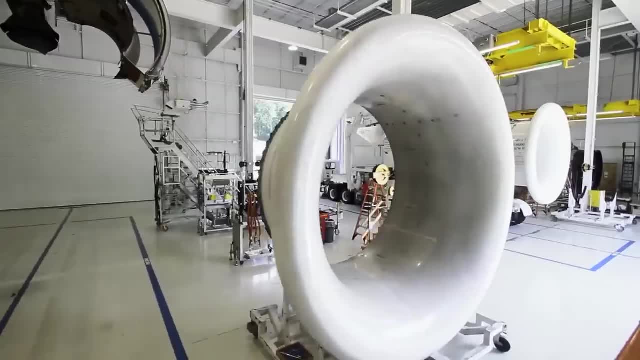 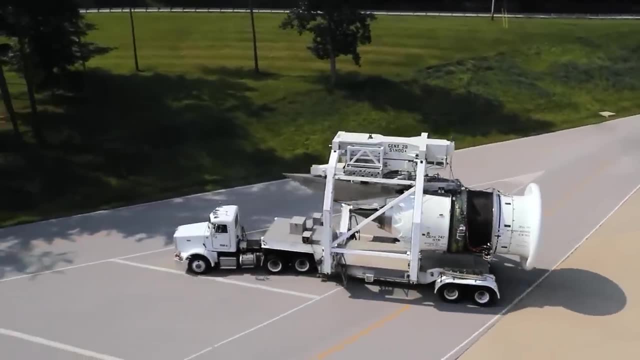 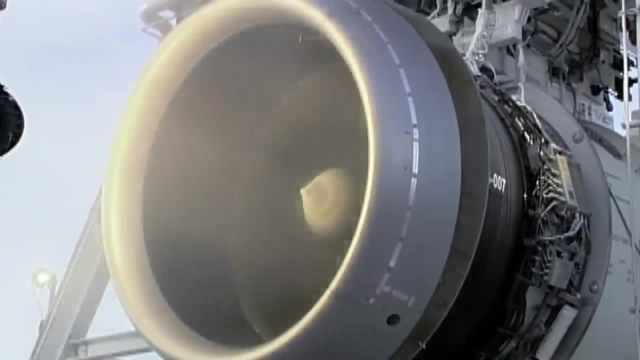 ratios. The reason for this is fairly simple: By increasing the pressure ratio we can maximise the energy we can extract from our fuel, Because there is more useful energy available for extraction in our turbine and nozzle than if we compressed the air less. But it's not quite as easy as just increasing pressure across our compressor. 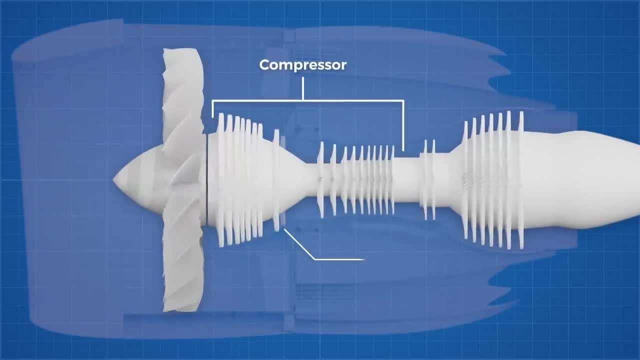 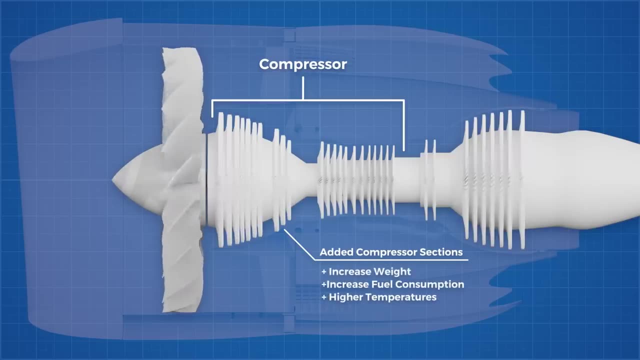 In order to achieve higher compression, we may need to increase the number of compressor sections, which will increase the weight of the engine, which will increase fuel consumption and reduce the advantage. Higher compression will also lead to higher temperatures, which may cause material failure in the compressor blades. 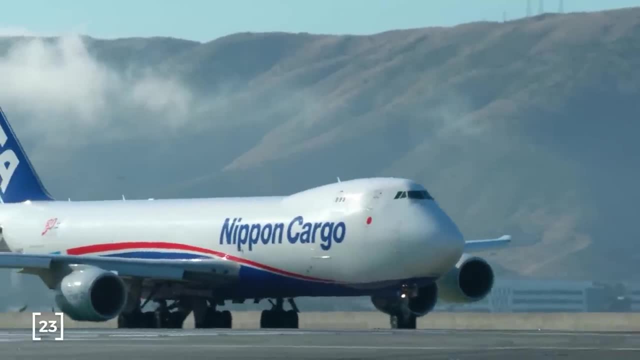 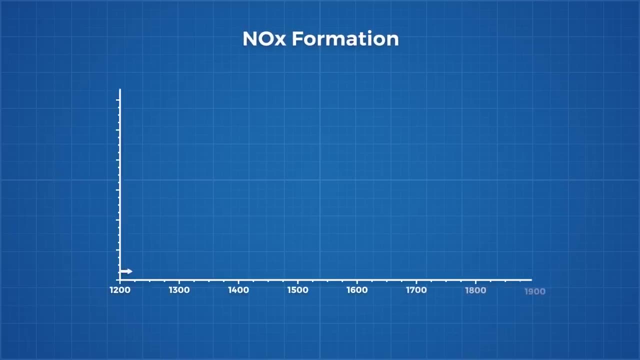 And perhaps most critically, increasing the temperature results in increased emissions of potent greenhouse gases like nitrogen oxides. Nitrogen oxide formation rates rise exponentially with flame temperature to break down nitrogen molecules in the air and allow them to combine with oxygen to facilitate increased pressure. 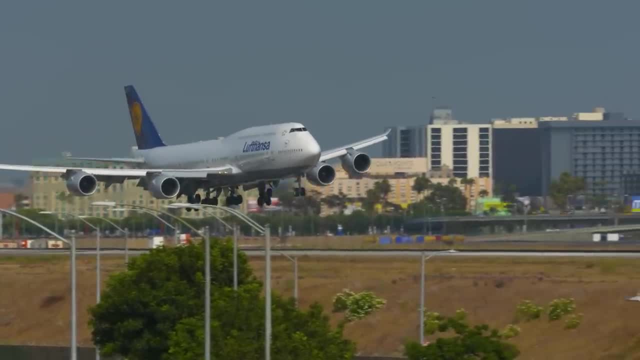 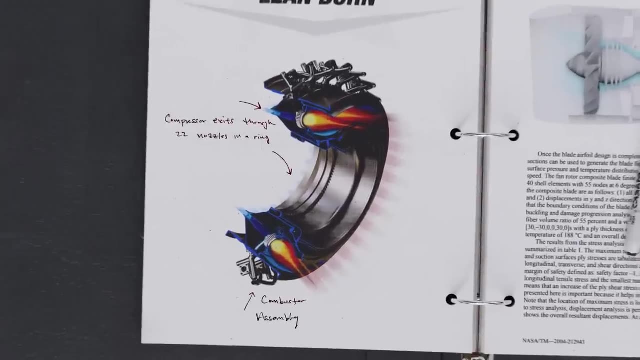 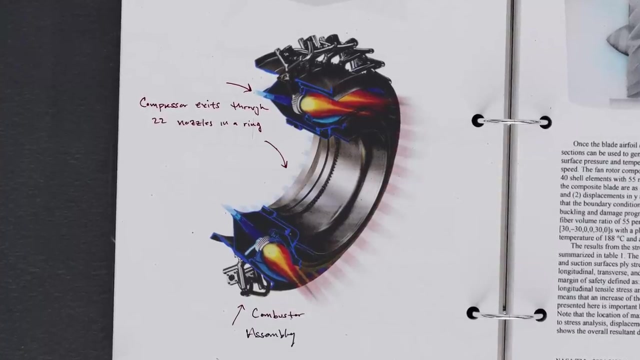 ratios While hitting climate change goals. this problem had to be addressed, and they did it through ingenious fuel injection technology. The compressor feeds its high pressure air into 22 fuel mixing nozzles located in a ring around the compressor exit. Their job is fairly simple: mix the fuel into the air and ignite it. 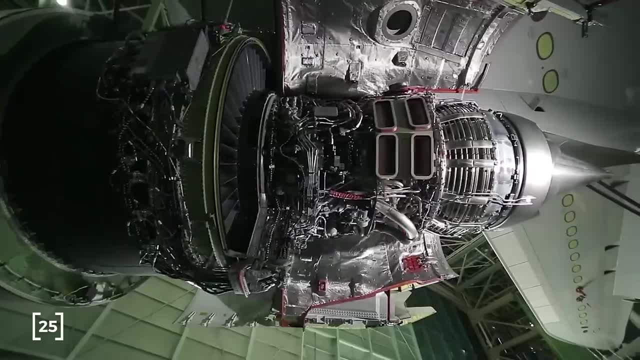 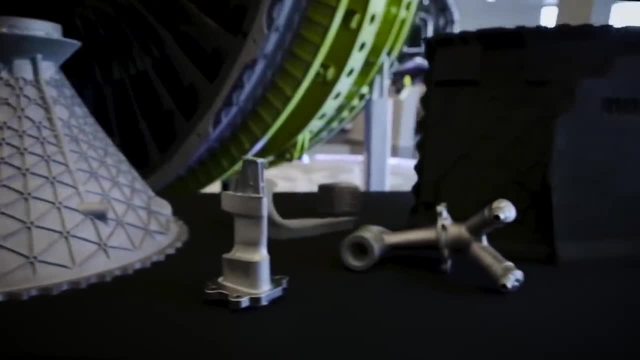 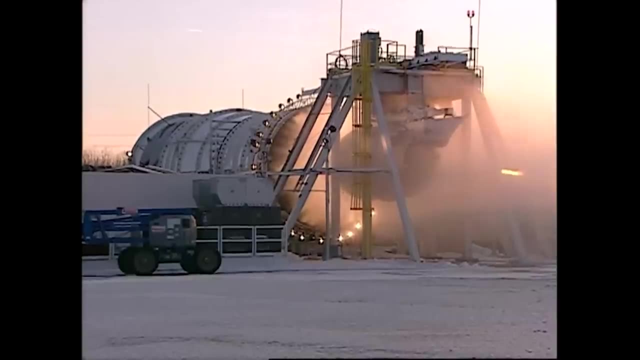 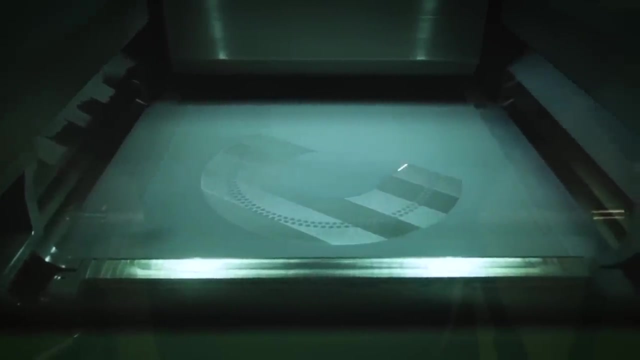 A simple job that started development in 1995 with both General Electric and NASA. The art of crafting the perfect fuel injection nozzle is incredibly complex, A delicate yet violent process, like an orchestra whose crescendo is a fiery explosion. With the advent of 3D printed manufacturing, GE has been able to create a fuel injector. 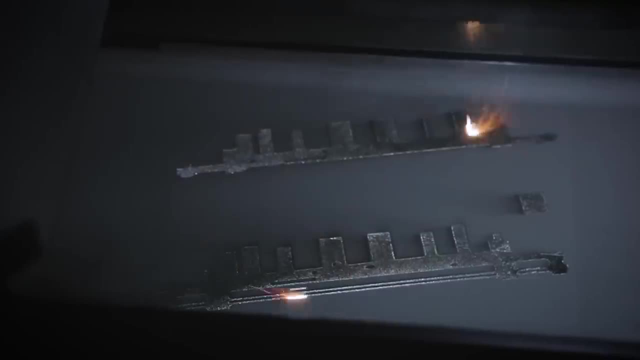 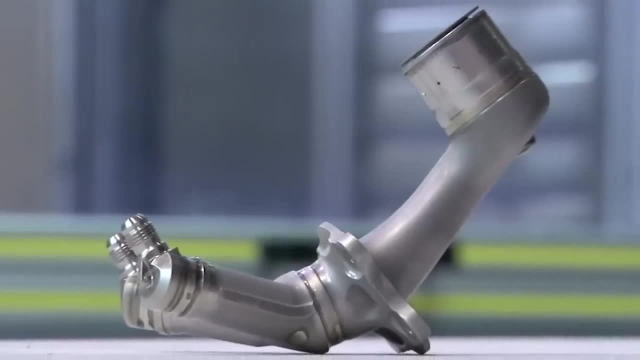 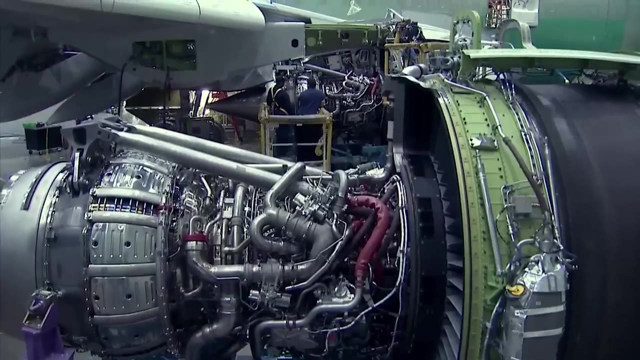 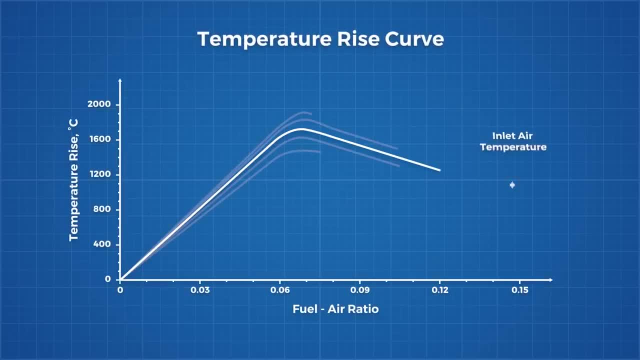 If we plot flame temperatures against air-fuel ratio, we get something that looks like this: The max flame temperatures occurring at stoichiometric air-fuel mixtures. That is the mixture where air and fuel are both entirely consumed in the reaction. This is the zone where nitrous oxide emits. 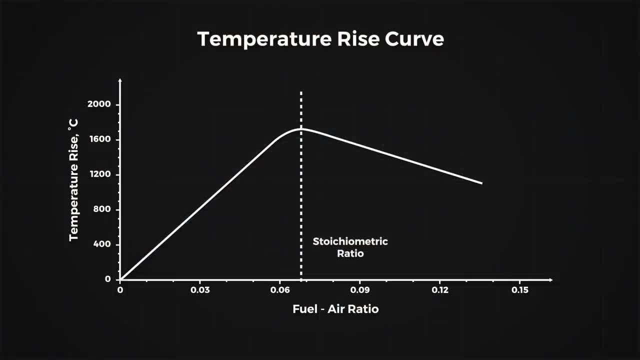 The. So instead we aim to be over here on the lean side of the graph. If we map the combustion process for GE's previous injector, fitted to over 22,000 CFM56, we would see the air-fuel mixture is initially injected in this zone with a rich air-fuel mixture. 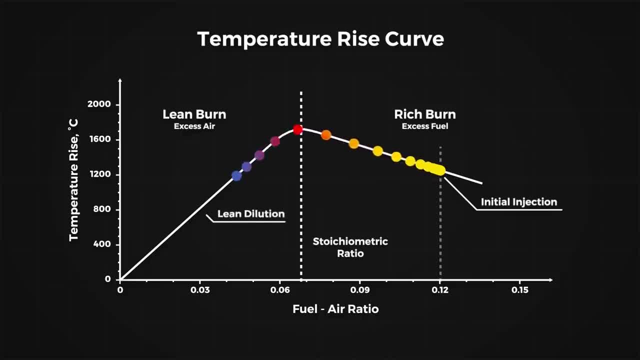 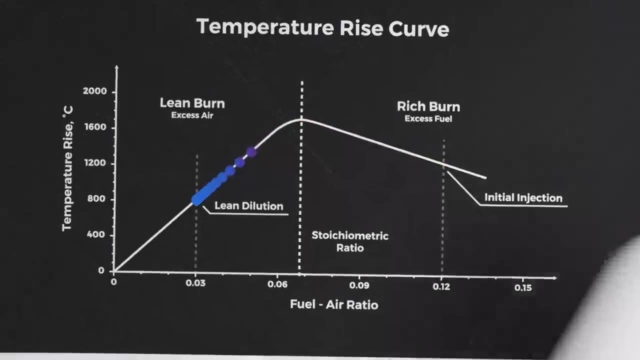 Then it goes through a dilution process to reach a lean mixture where the fuel is fully consumed. The issue with this is that the fuel goes through the stoichiometric region in between these two phases, creating a great deal of nitrous oxides. The TAPS fuel injector looks like this, with the central main pilot surrounded by a ring. 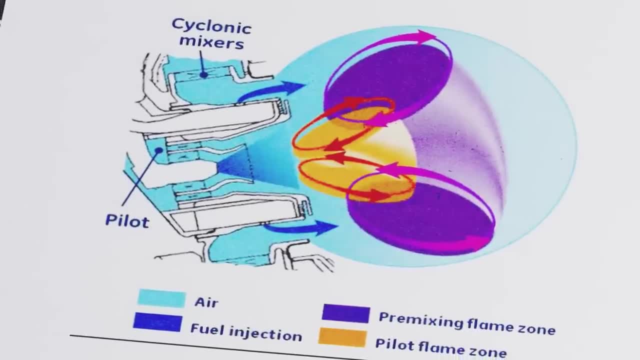 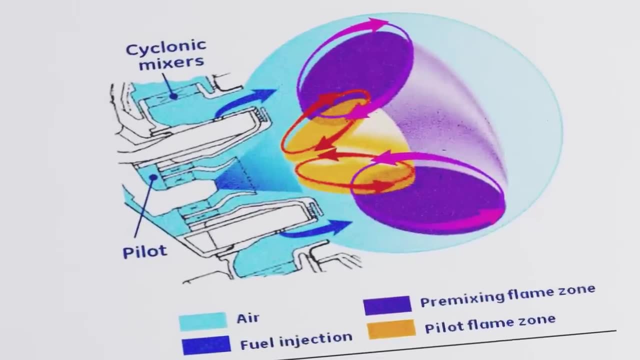 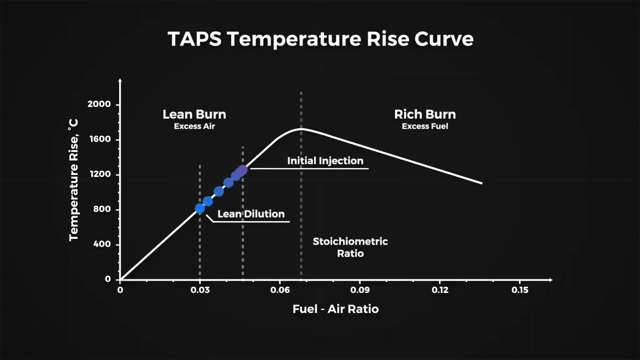 shaped main injector Creating two swirling air flows that looks something like this, Which uses a large amount of air in the pre-mixing phase to ensure thorough mixing and a lean air-fuel mixture. If we map the combustion process of TAPS, it starts in the lean zone and gets even leaner. 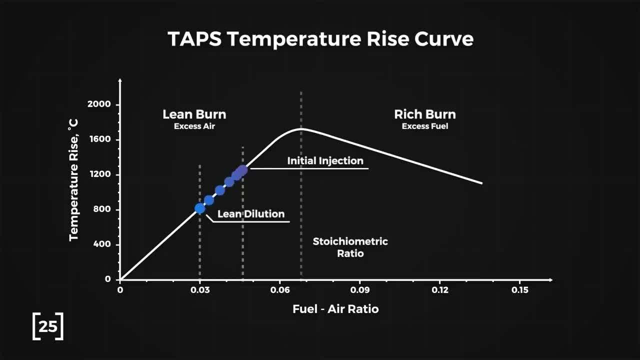 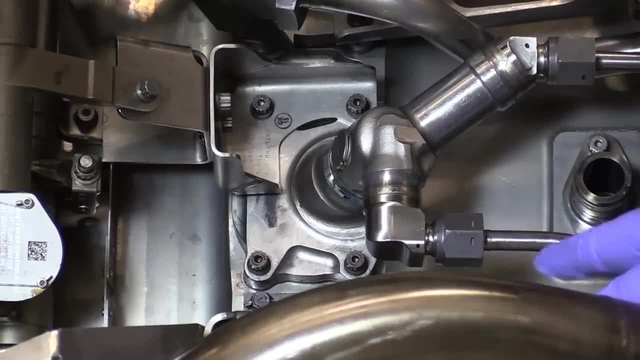 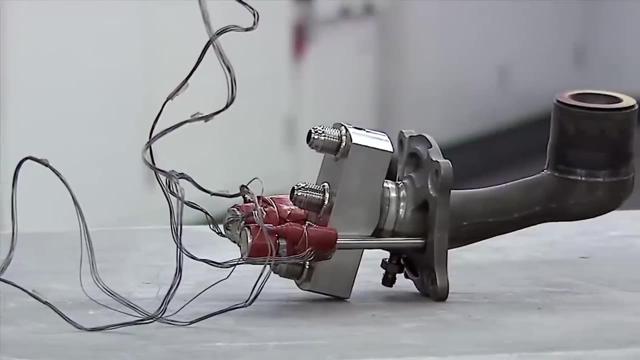 further into the combustor, never getting close to the peak nitrous oxide production region. This may seem like a simple device, But it took generations of design iterations, with computer simulations gradually bringing the engineers closer to their target, And none of their designs would have been possible without current generation metallic. 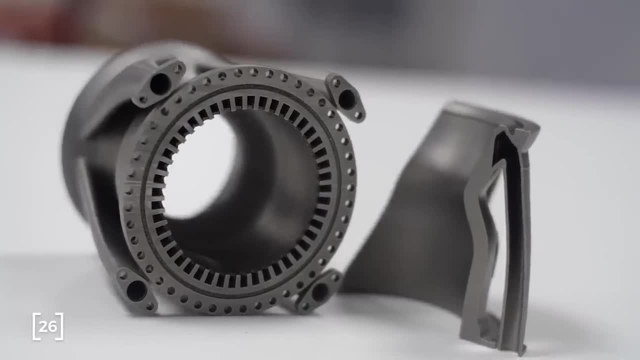 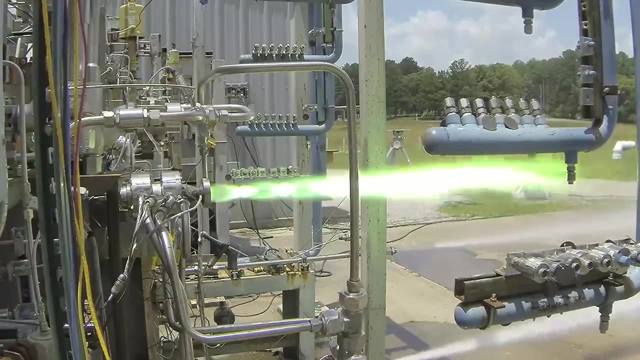 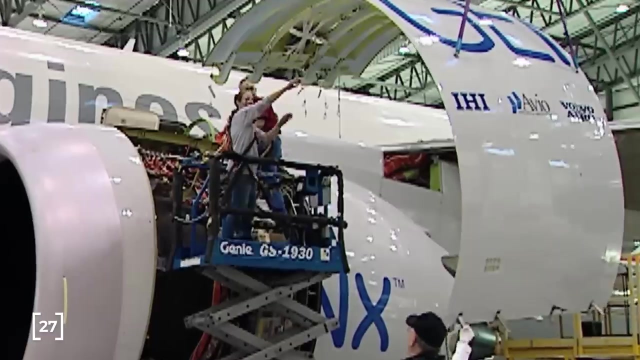 3D printing that could manufacture the complex parts with the materials capable of resisting the enormous heat within the combustor. 26 years of development paid off with 60 percent nitrous oxide emission reductions. A fuel injector compatible with the record breaking 58 to 1 pressure ratio used in the GE NX. 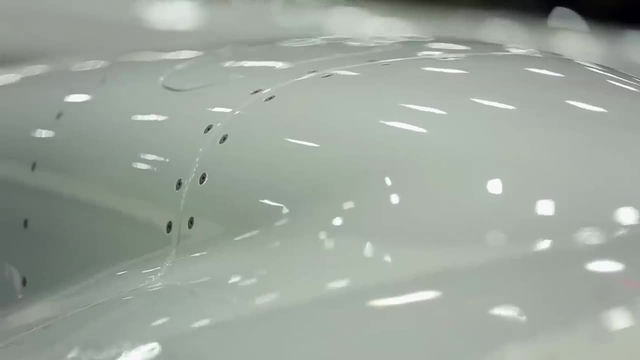 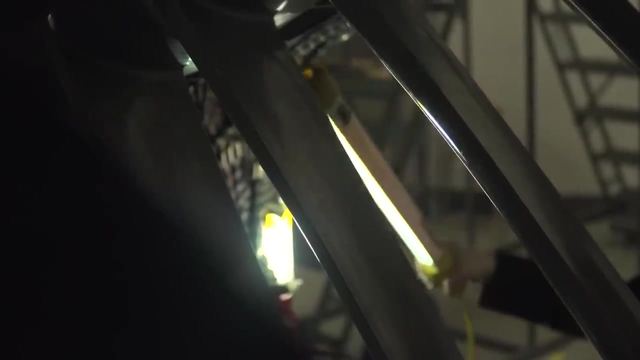 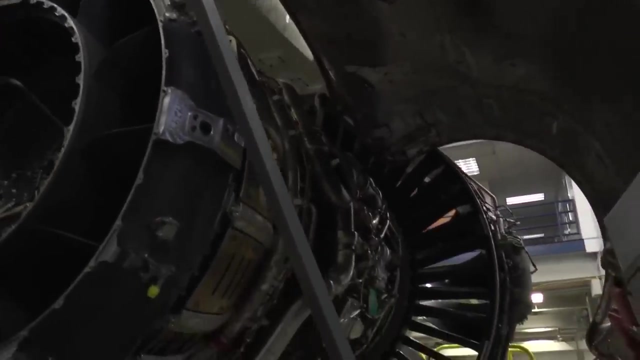 GE managed to increase the pressure ratio, even though they reduced the number of compressor stages. Each of these turbine discs is one stage. The GE NX contains 10 stages, Four fewer than the CF6 engine it is replacing. GE managed to do this through new, improved blade design. 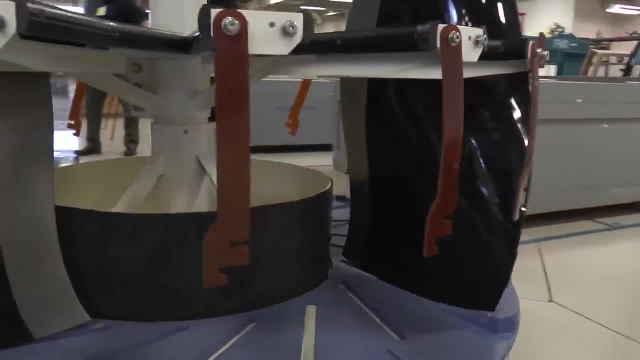 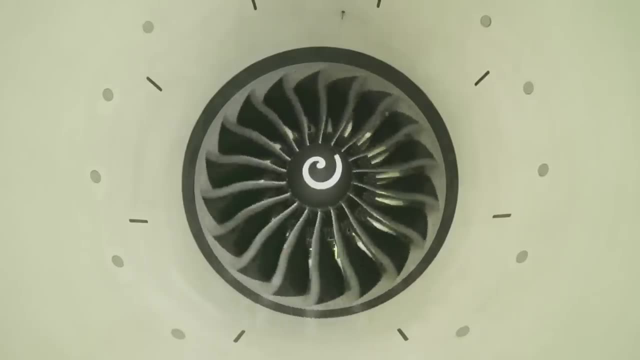 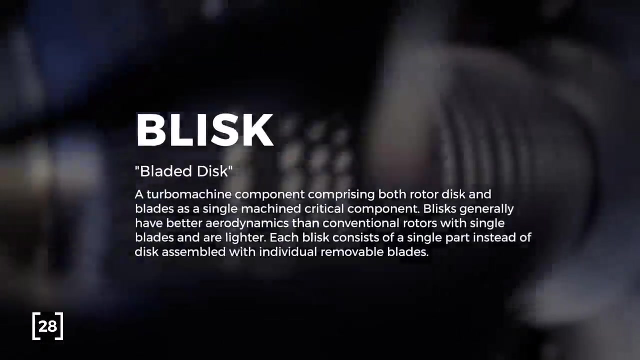 Which is a lot less info than I wanted to share, but finding information on this topic was incredibly difficult, A testament to how advanced and secretive the technology is. The compressor does include three blisk stages, which are perhaps the most impressive feats of machining I have ever seen. 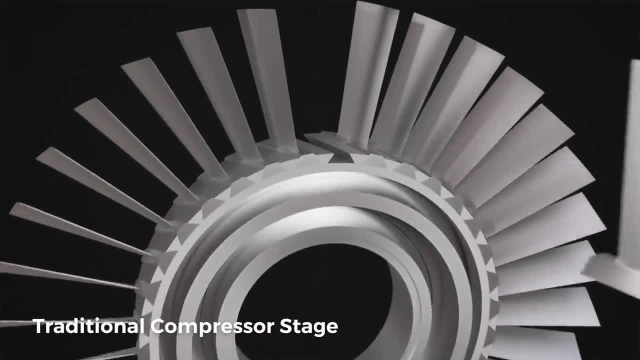 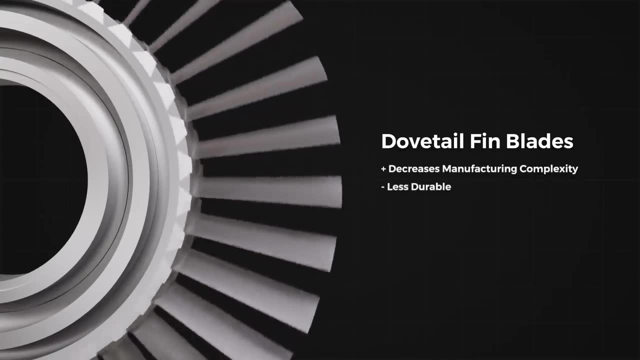 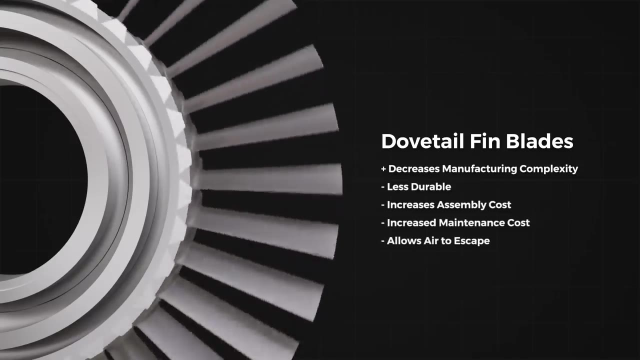 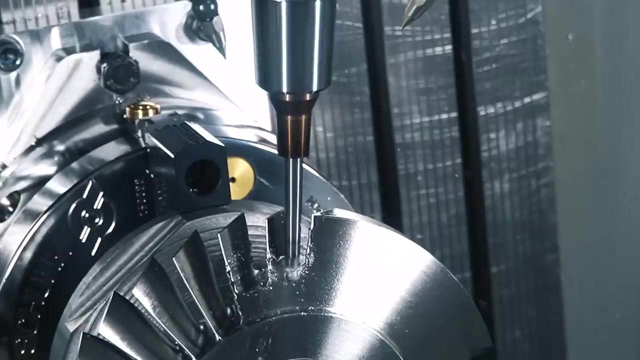 Traditionally, compressor stages are made by attaching the blades to a separate disc with dovetail connections. This decreases manufacturing complexity, but the dovetail connection is less durable, increases assembly and maintenance costs and allows some air to escape through the connections. Blisks are compressor stages that are manufactured from a single piece of metal making them. 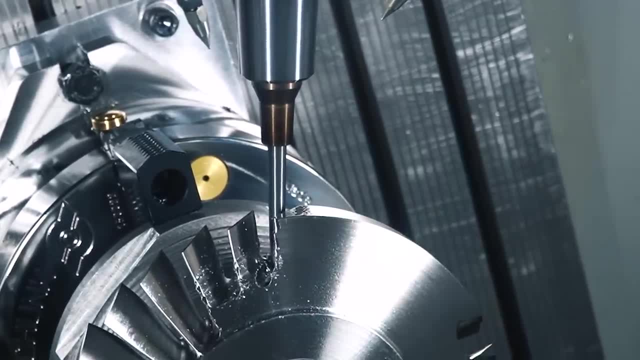 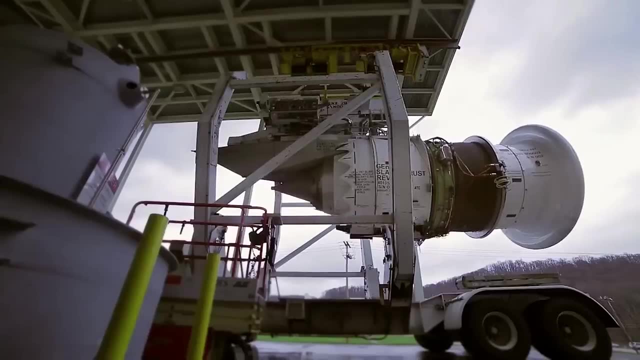 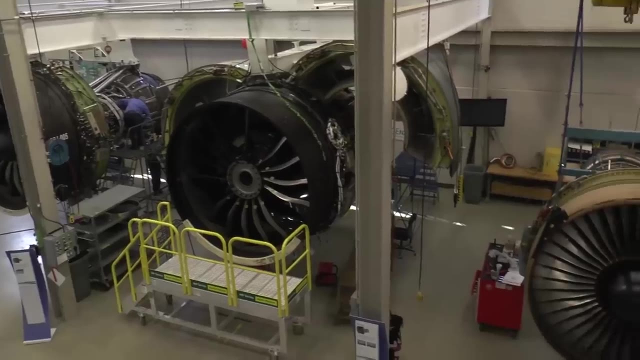 stronger and easier to install, while improving aerodynamic efficiency- Improving aerodynamic efficiency was the name of the game- to improve compression ratios and of course, that needed to apply to the turbine section that powers the compressor. It, too, benefitted from cutting edge aerodynamic modelling. 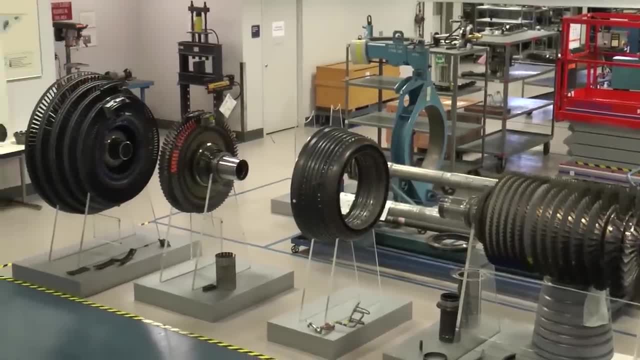 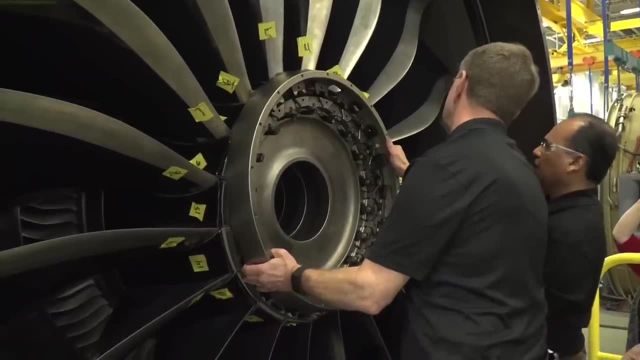 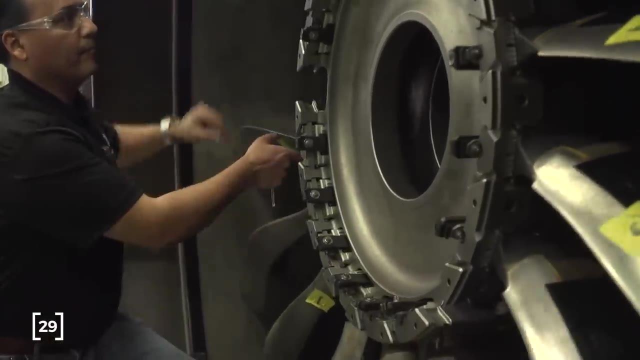 The turbine also made use of new material science breakthroughs, being the first commercial engine to make use of gamma titanium alumini, An advanced alloy of titanium and aluminium that combines the heat resistance of titanium with aluminium's weight savings, replacing the nickel alloys of past. 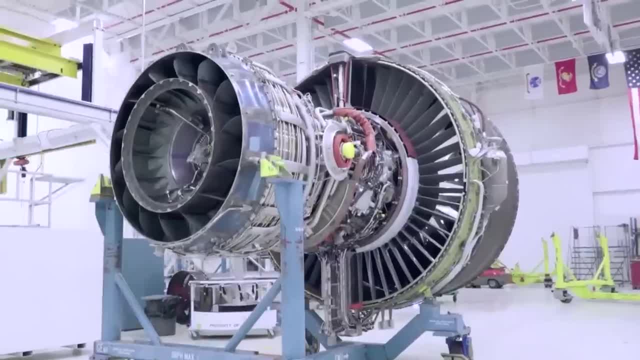 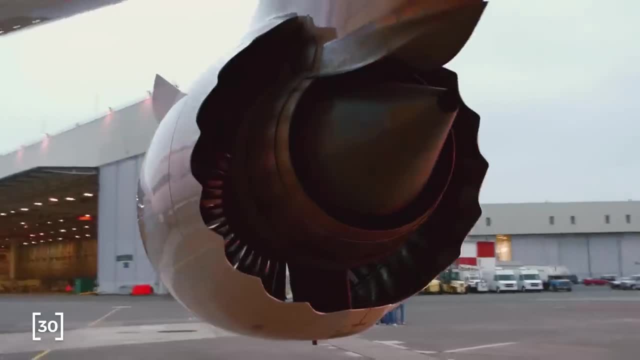 It took three decades to make this engine. It took a lot of work. It took decades to take this material from the lab to commercial use And the Dreamliner was the first plane to make use of it, paving the way for the materials acceptance in the industry. All of these factors combined to allow the GENX engines of the Dreamliner to reduce fuel consumption by 15% over previous generation engines. That is an astronomical leap, and on top of all, that the engine is 60% quieter than similar sized planes. 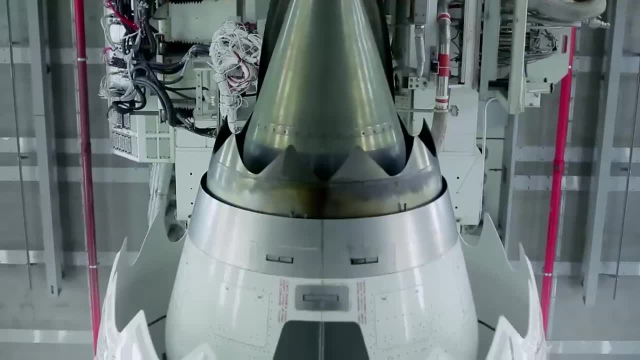 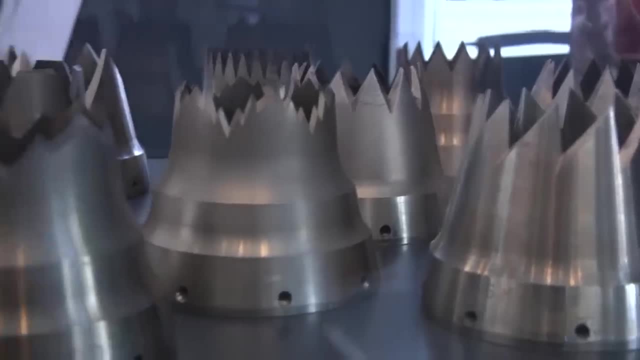 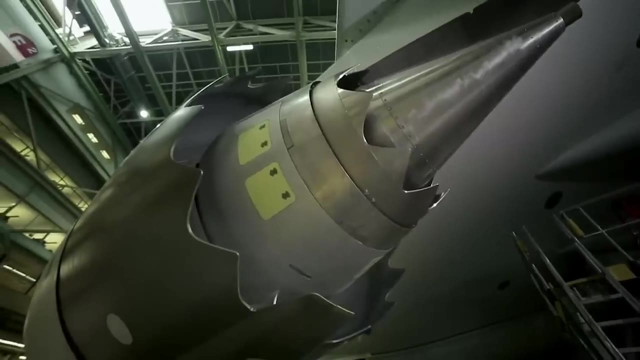 In part thanks to the engine's most distinctive feature, This sawtooth pattern on the fan casing and the engine exhaust. These features are called engine chevrons, and they aren't just futuristic cosmetic design, but functional parts of the engine that significantly reduce engine noise. 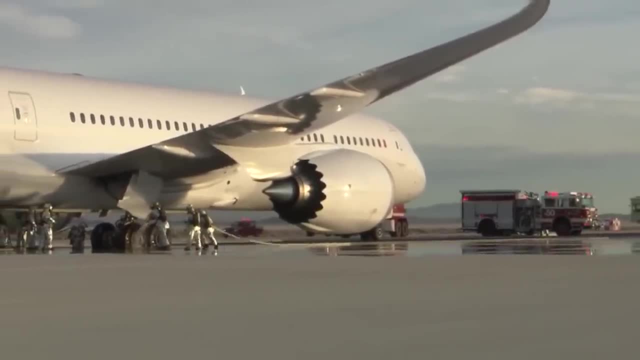 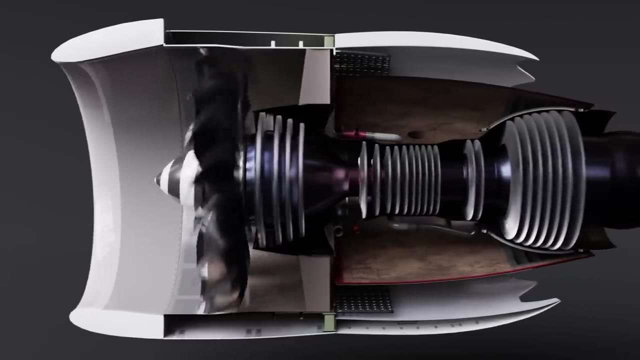 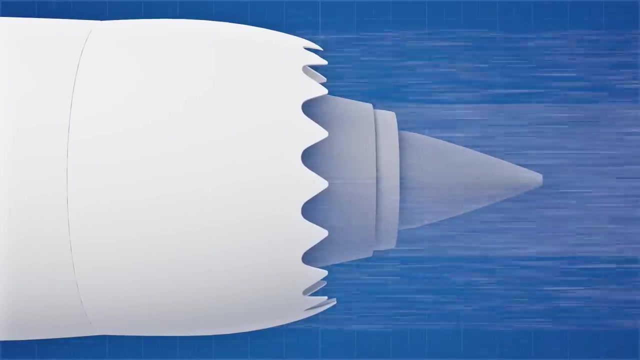 The question is: what difference can a mere shape change at a nozzle exit have on the overall noise pollution produced by the aircraft, Because turbofan engines force air out of their bypass chambers and turbines at speeds that are much higher than the speed of the ambient air. 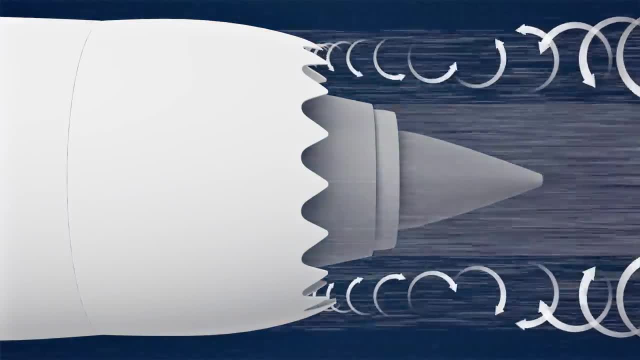 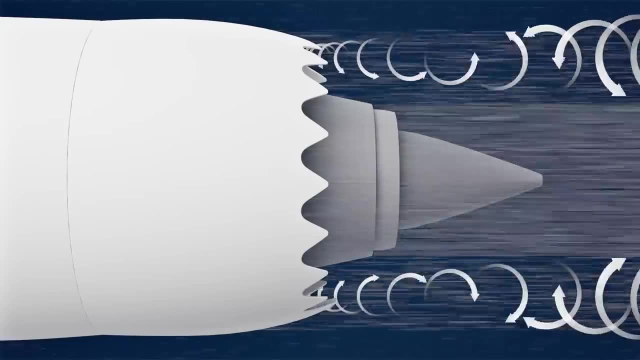 The air interacts with the freestream air, causing mixing. This mixing causes uncontrolled vortices, which in turn generate excessive noise for both the passengers and the community on the ground. Think of it like water accelerating down a waterfall and striking the water below. 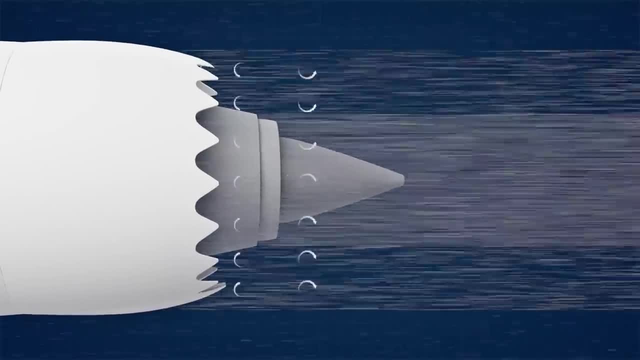 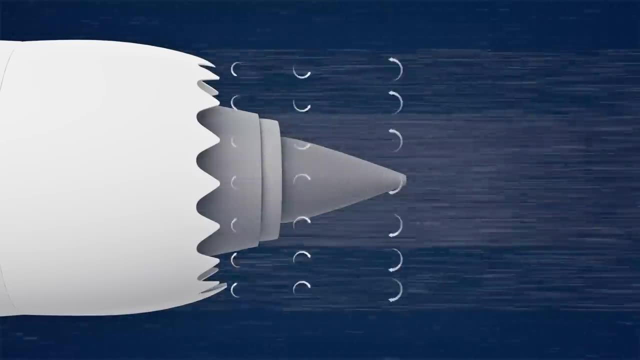 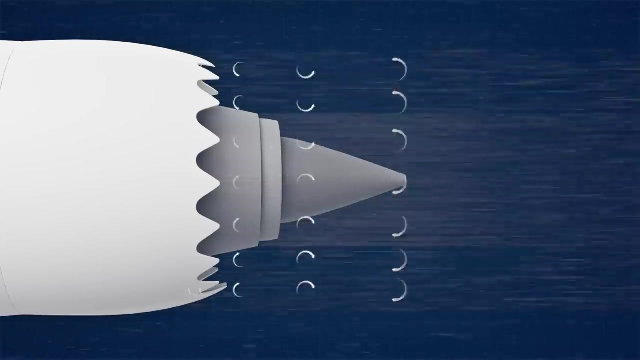 That turbulence can be extremely loud. The chevrons aim to control the vortices that are shed from the engine nozzle by creating smaller vortices at each of the teeth of the chevron to allow the hot, fast air being expelled from the engine to mix with the ambient air more gently. 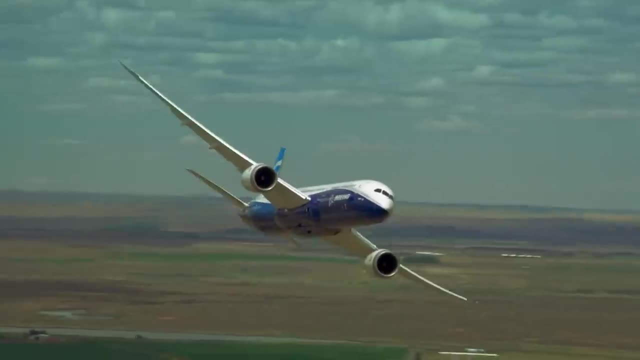 This is said to reduce jet blast noise by as much as 30% and allowed Boeing to use substantially less sound insulation in the fuselage walls of the aircraft. This is said to reduce jet blast noise by as much as 30% and allowed Boeing to use 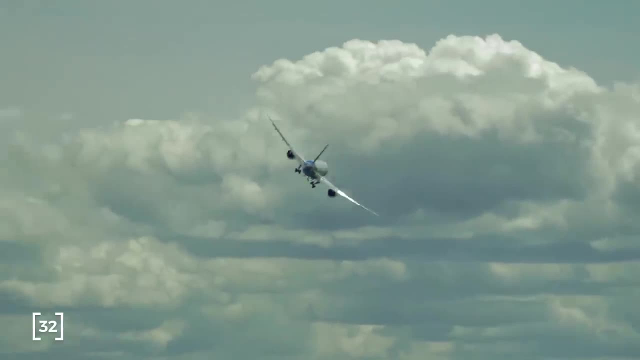 substantially less sound insulation in the fuselage walls of the aircraft. This is said to reduce jet blast noise by as much as 30% and allowed Boeing to use substantially less sound insulation in the fuselage walls of the aircraft. This is said to reduce jet blast noise by as much as 30% and allowed Boeing to use substantially 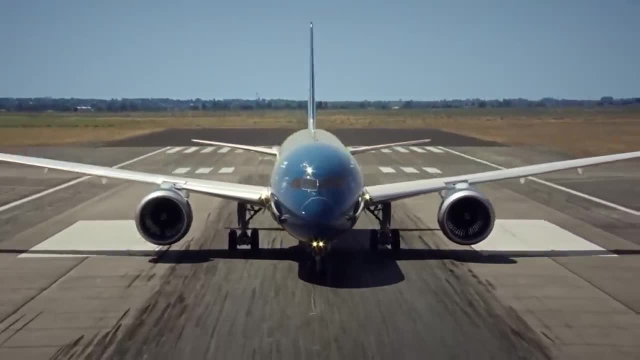 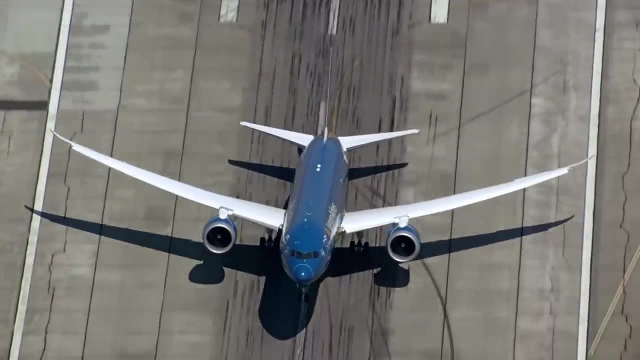 less sound insulation in the fuselage walls of the aircraft. The 787 truly does live up to its name. It provides a passenger experience that is almost incomparable to that of other commercial aircraft, with advances in noise reduction, fuel efficiency and passenger comfort. 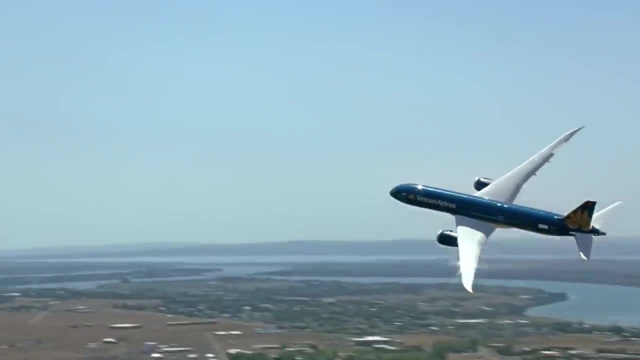 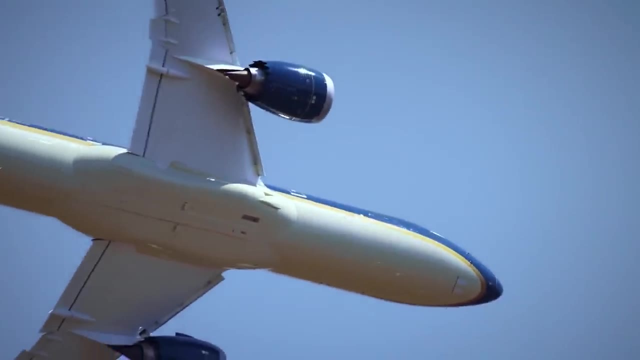 This series is usually saved for aircraft and technology most of us will never set foot in, But the 787 could be the most advanced piece of engineering we have ever covered. The 787 could be the most advanced piece of engineering we have ever covered. 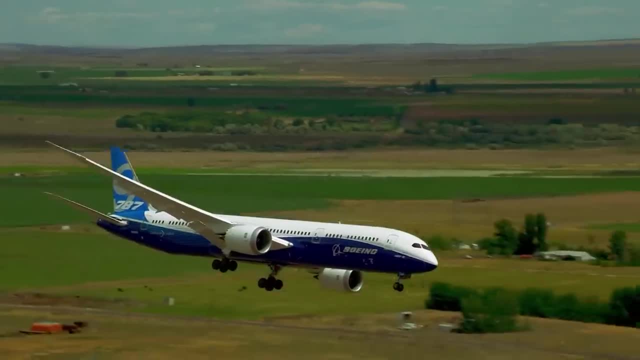 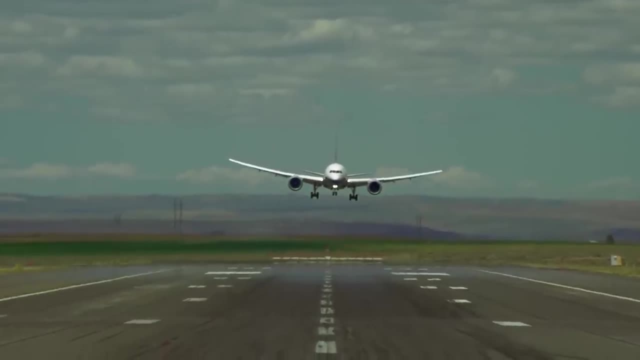 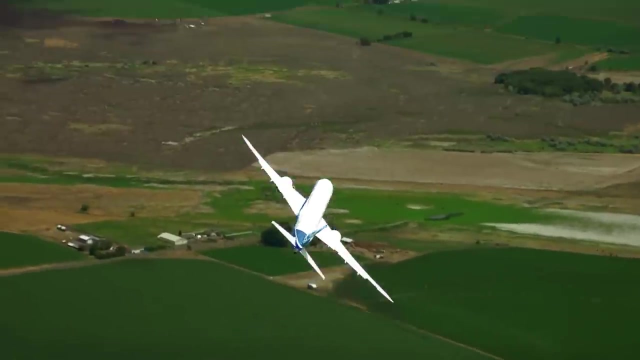 And it's a plane many of us will have the opportunity to fly in and marvel at the decades of engineering advancements that made it possible. This nearly half hour long video is just half the story, but the full hour long director's cut version has been available on Nebula for over a week. 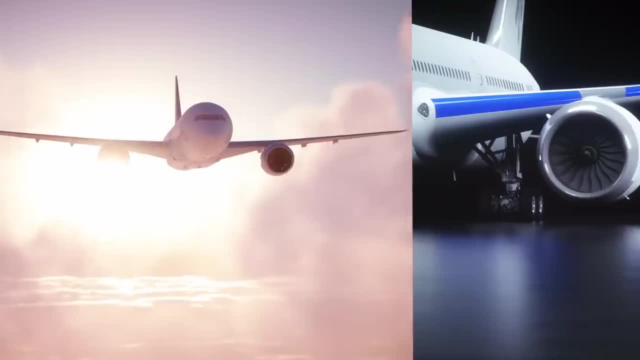 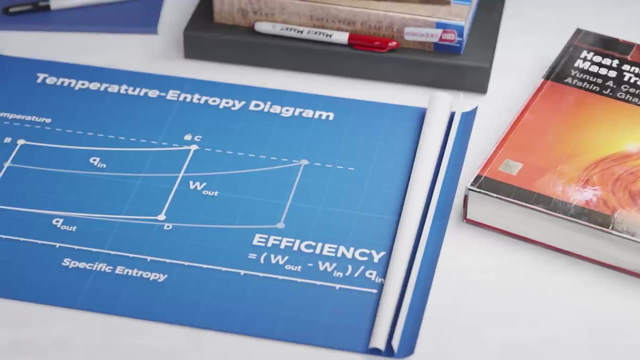 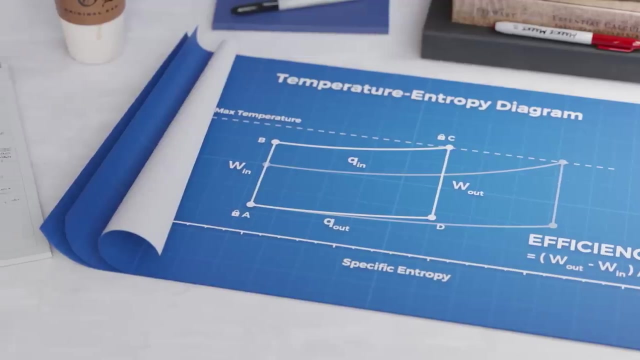 It combines the two halves of this video released on YouTube into one seamless ad free experience that you can sit back and relax and enjoy. Thanks for watching. I removed one section from this video detailing the complicated thermodynamics explanation of why compression ratios actually increase efficiency because it felt just too academic. 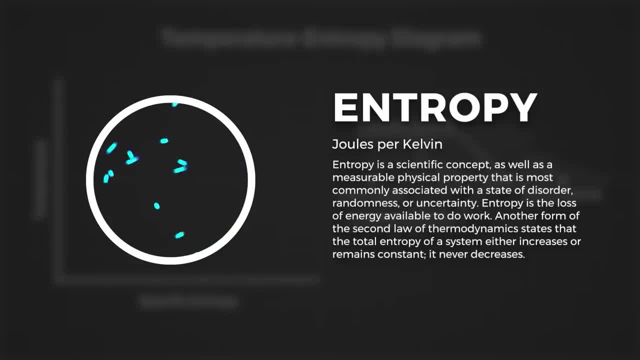 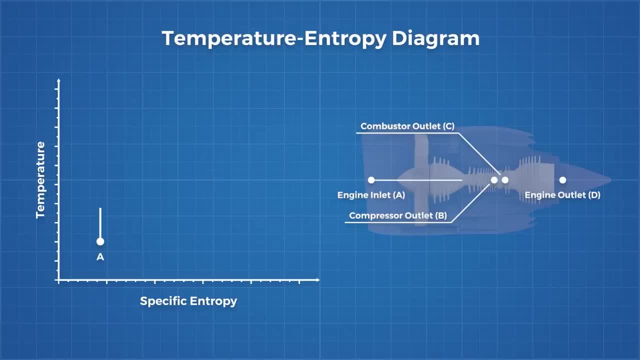 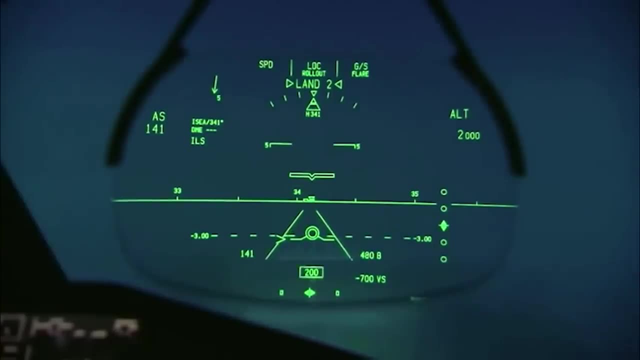 for YouTube, But I think die hard fans of this channel may enjoy listening to a 10 minute explanation of temperature entropy diagrams. The director's cut also includes explanations of the 787's nifty electronic headlight, heads, up display in the cockpit and electrochromic window shades. 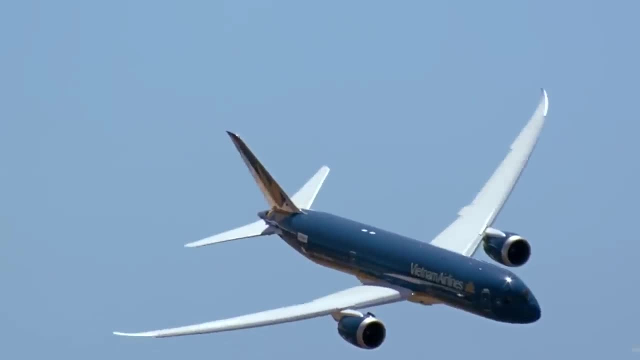 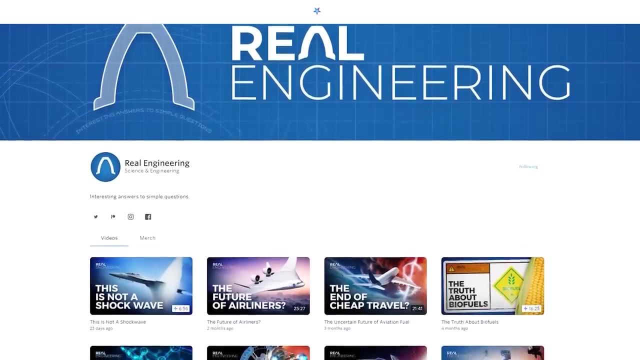 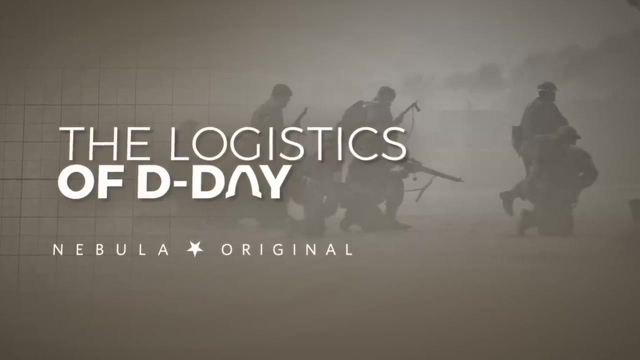 I felt neither of these topics really fit in anywhere in the larger script. Nebula is the best way to experience our videos: No ads, no distractions and director's cuts of videos when possible, along with exclusive access to our World War 2 series, The Logistics of D-Day and our upcoming Battle of Britain. 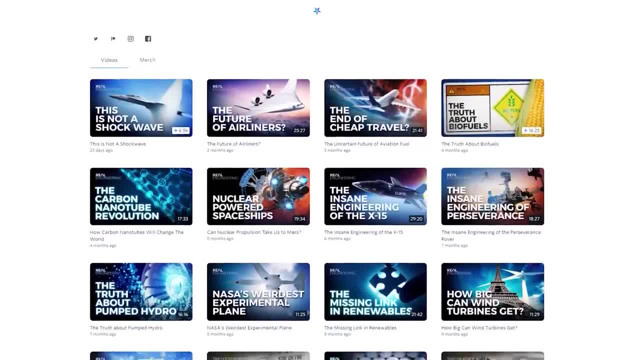 series. If you want to see more content like this, the best way to support our channel is by clicking the link in the description of this video. If you want to see more content like this, the best way to support our channel is by clicking the link in the description of this video. 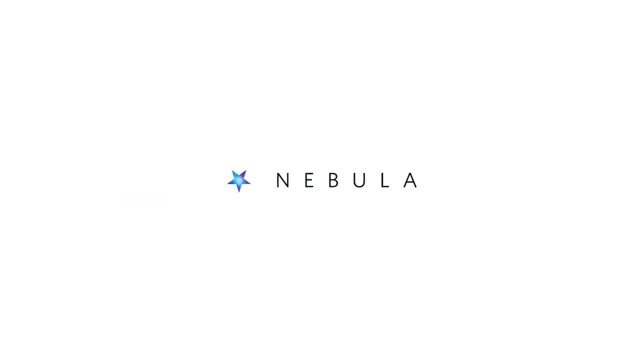 If you want to see more content like this, the best way to support our channel is by clicking the link in the description of this video. If you want to see more content like this, the best way to support our channel is by signing up to Nebula with the Curiosity Stream Bundle. 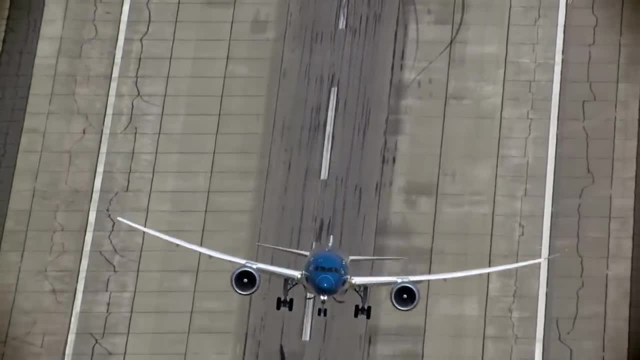 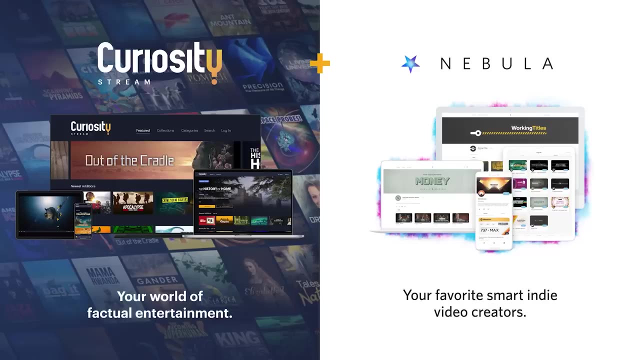 I've included a link to the director's cut in the description. for those of you already subscribed to Nebula or if you've yet to start supporting the channel there, you can sign up through the Nebula and Curiosity Stream bundle deal for just $14.79 a year. that's. 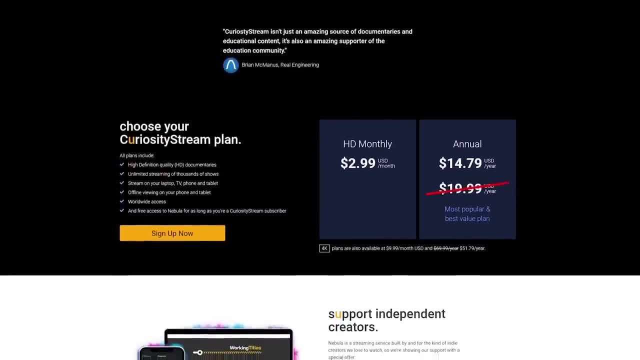 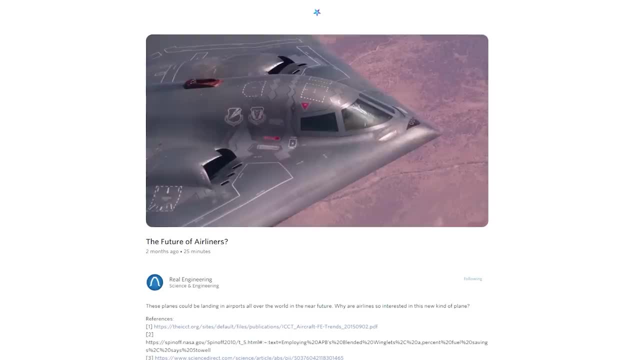 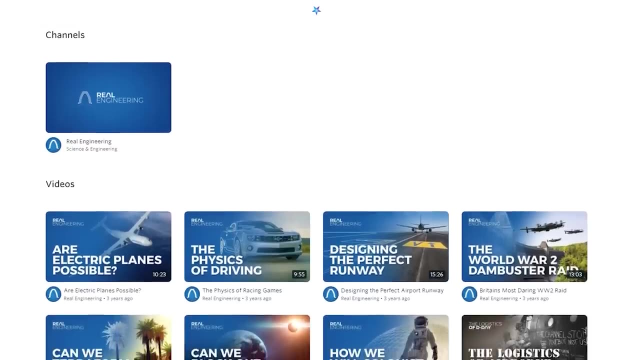 over $1 a month, But that one dollar has a gigantic impact on this channel because we get to own and run our own streaming platform and that gives us the freedom to create what we want how we want. A little over $1 a month, this is by far the best way to support. 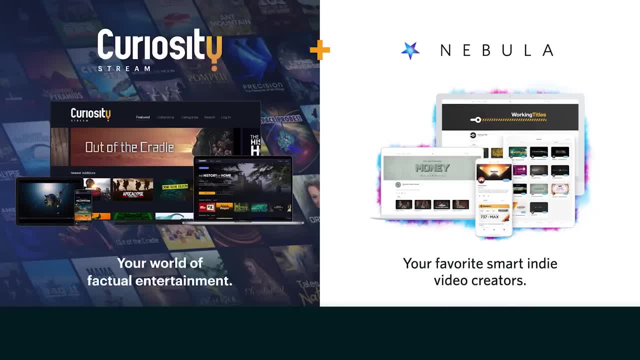 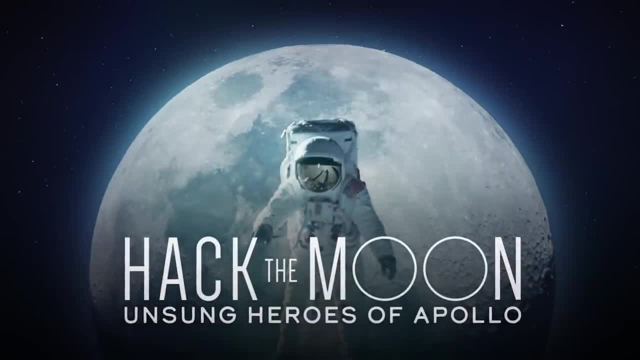 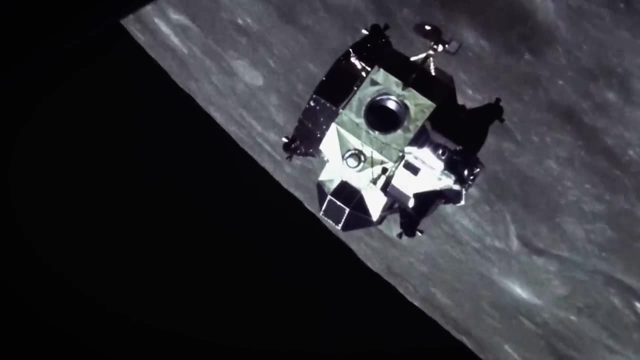 this channel and get something in return, with access to both Nebula and all the amazing award winning documentaries on CuriosityStream, Like this one called Hack the Moon, about the fascinating technologies engineers developed for the Apollo Moon mission. You can sign up to this. 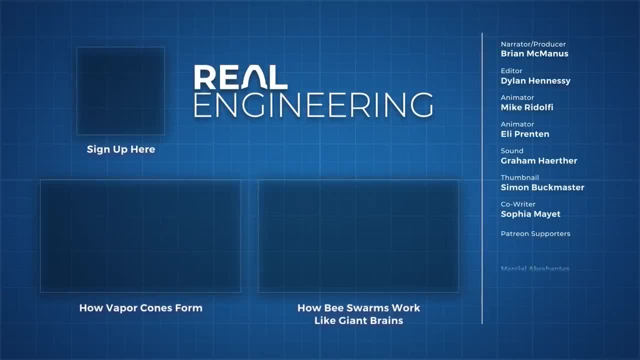 amazing deal by clicking on this button on screen right now, Or if you are looking for something else to watch. right now, you could watch our last video on how vapor cones form on planes. Or you could watch Real Science's latest video on how bee communication is helping us learn about the brain.